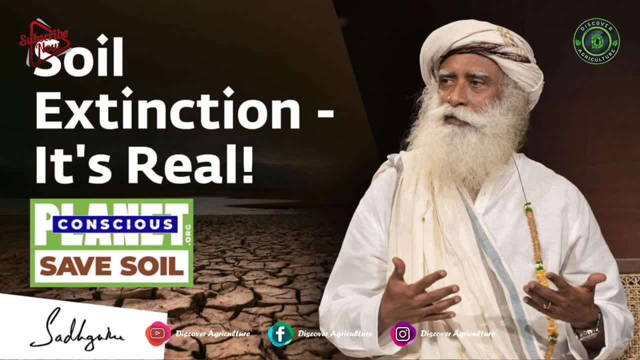 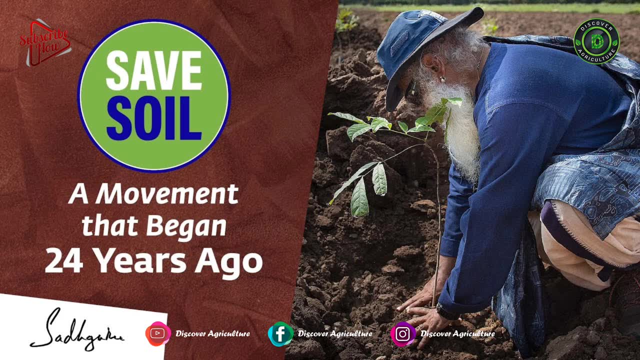 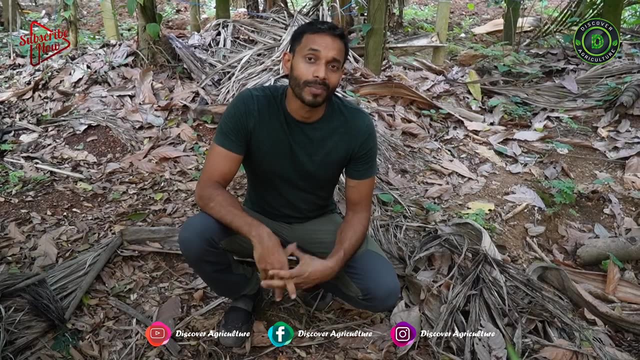 Now we all know that we have seen Sadhguru from India traveling around the world talking about the life, life, the health of soil, and he's on this mission to save the soil. so he's talking nothing but how we are losing this soil microbiology, the species- about 27,000. 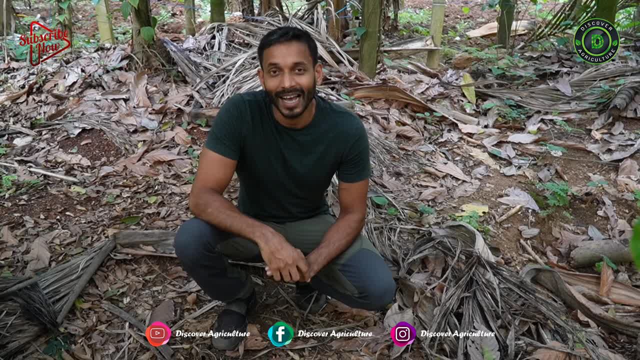 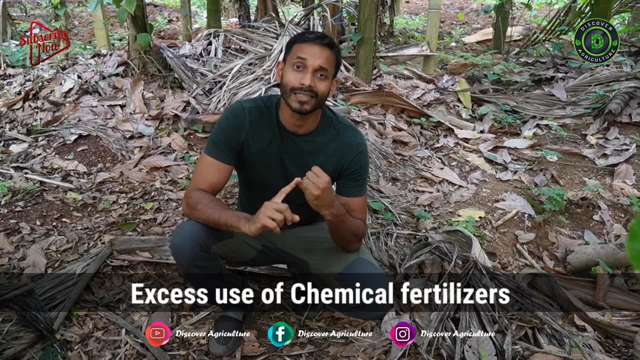 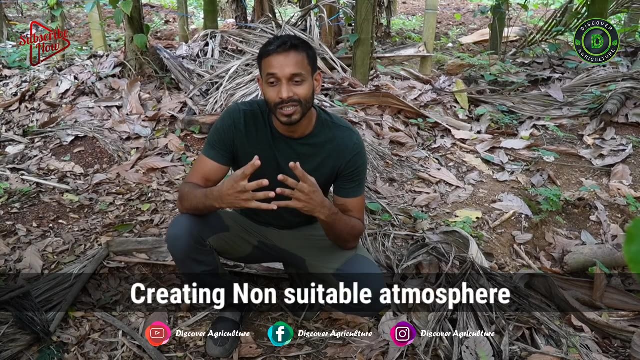 different species of soil microbiology we are losing per year, and the planet as these. this is happening due to various reasons. one is excess use of chemical fertilizers. the other one is doing motor culture and basically creating an atmosphere which is not suitable for the flourishment of microorganisms. so now 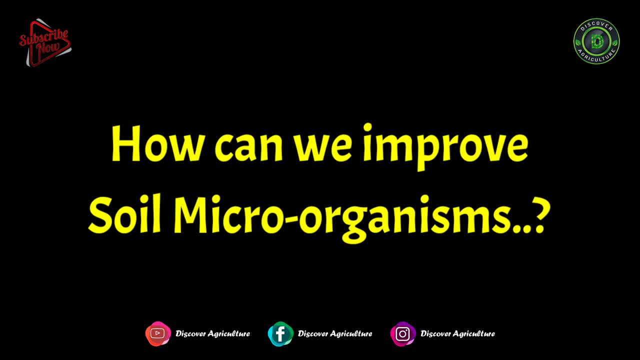 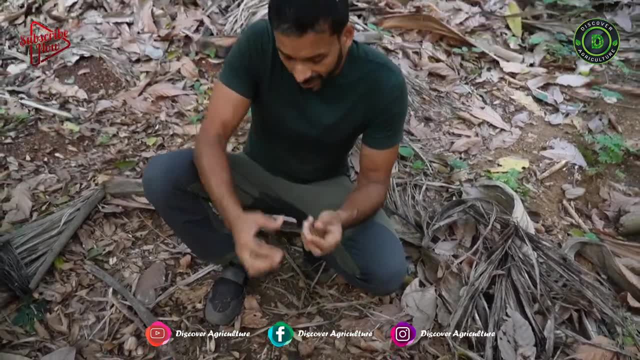 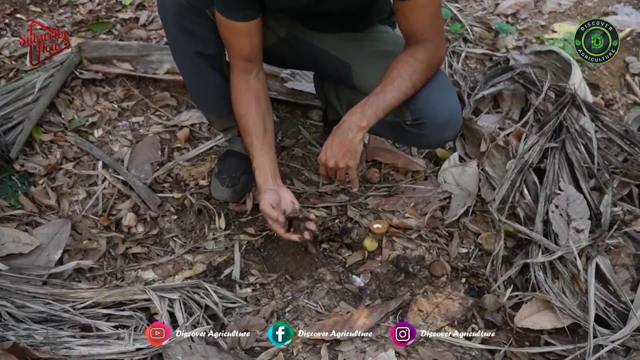 let's talk about how we can improve the microorganisms, so these microorganisms which basically degrade the organic matter back into the soil. as we can see, the organic content in the soil is so high and this is because of pl? ws. kaikki o vaccine? oagen is Miranda P? そう porch 쓰�人陸幹. 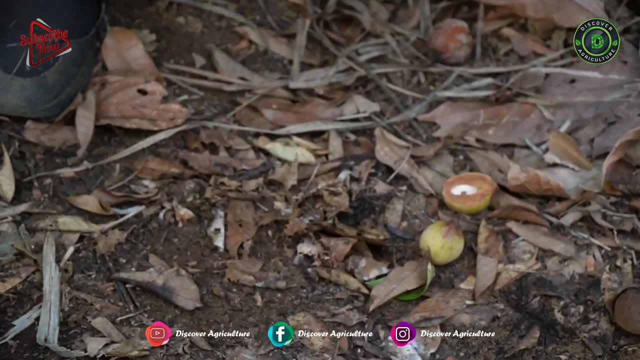 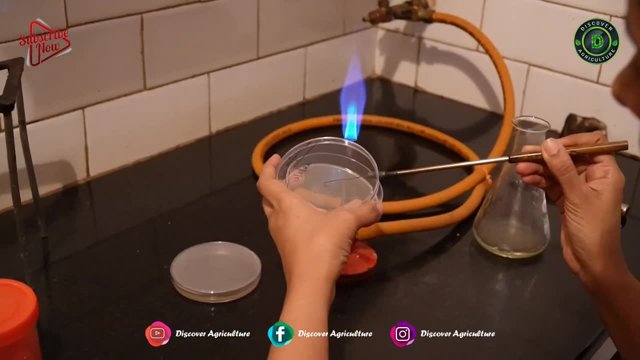 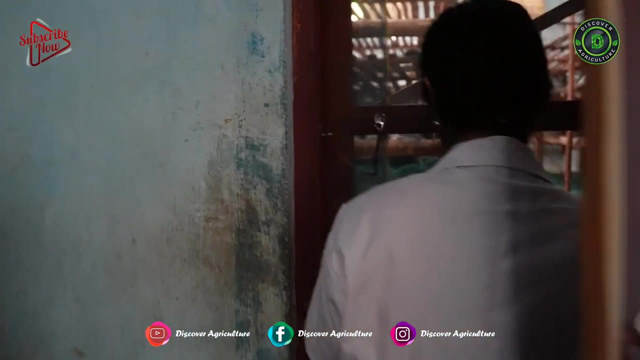 presence of all the different organisms here. so how? what we can do, like what we have done at at our farm for the last 30 years, with the help of our research center in Varanasi Development and Research Foundation, we have isolated certain microorganisms which are highly beneficial for the plants. there are the 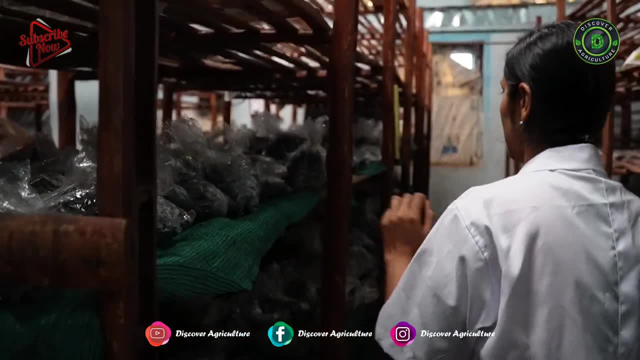 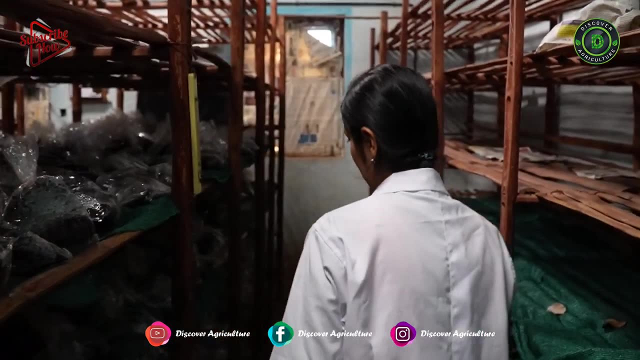 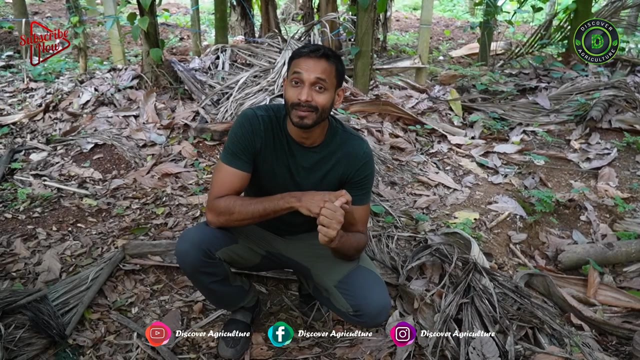 nitrogen fixers, there are the possible solubilizers, the potassium mobilizing bacterias, and there are biocontrol agents and there are microorganisms which produces, like bacteria, which produces plant growth hormones, and they produce the secondary metabolites which improves the immune system of the plant. 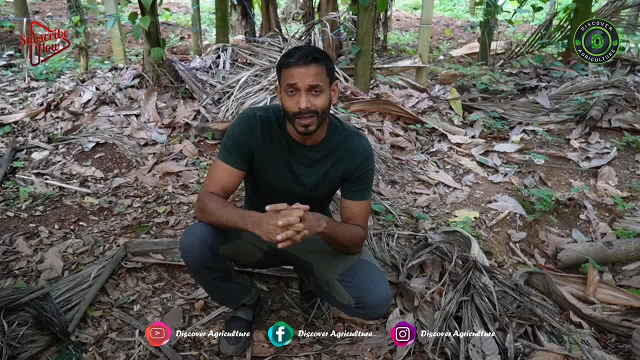 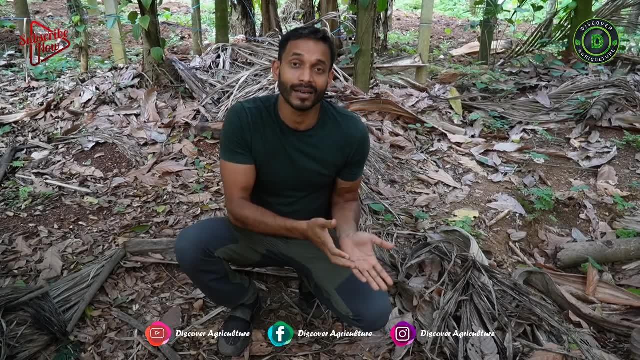 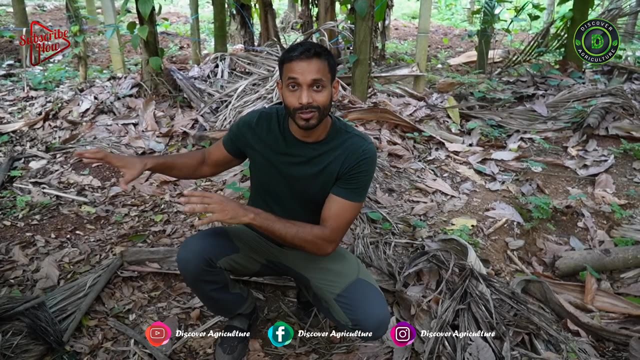 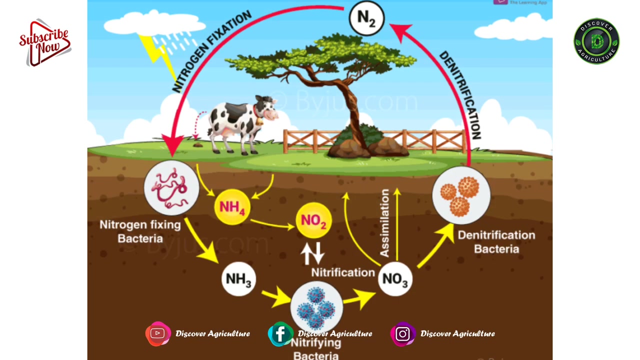 so there are these various organisms that they are present in the soil, which are championing the symbiosis between plants and and the soil. So in their presence they keep the bad pathogens away, they help the degradation of nutrients and make it bioavailable for the plants, giving you 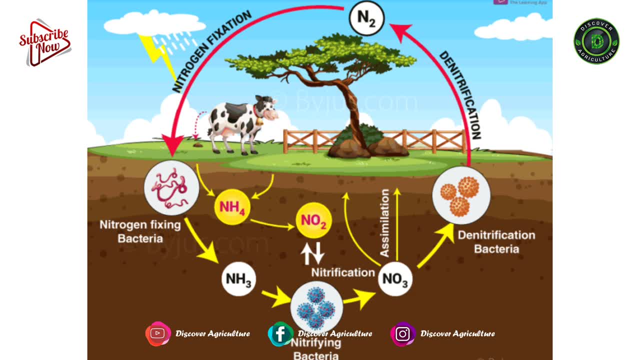 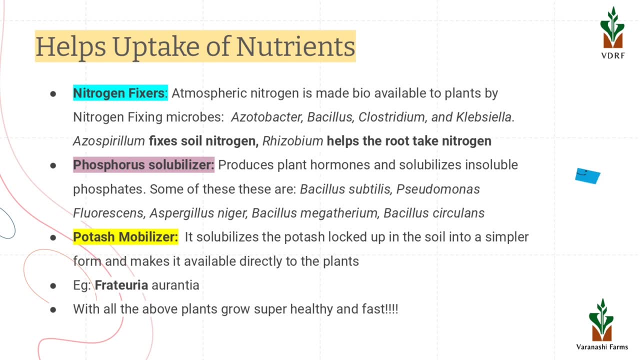 an example. you know the. things like nitrogen needs to be fixed into the soil, into bioavailable form. Phosphorus can easily react with cations such as of like iron, magnesium, zinc and form complexes which are not available for the plants to be absorbed. 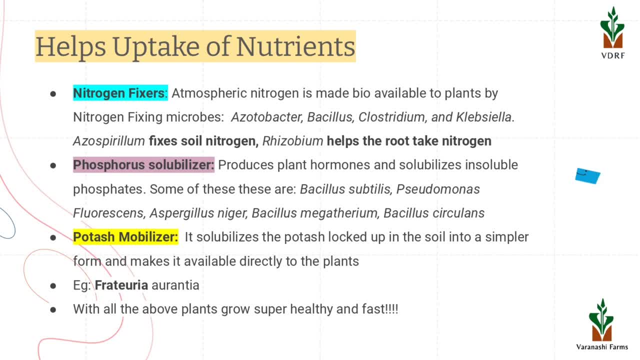 So these microbes? they release certain enzymes which break down these complex molecules into simple form of nitrogen, phosphorus and potash, which is, and also the microbes and the secondary nutrients which are readily absorbed by the plants. so this is why the presence of microorganisms is very, very essential in 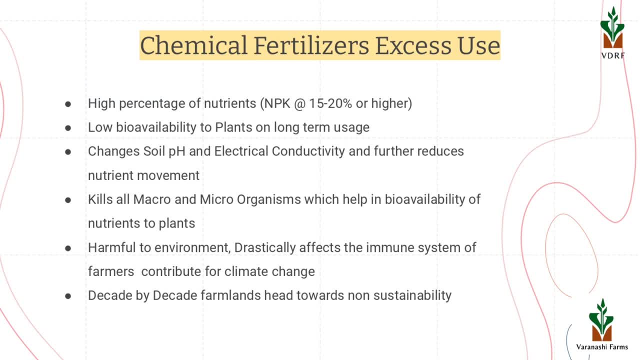 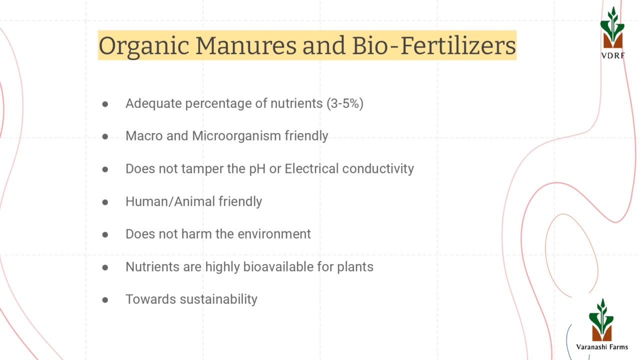 the in our farm just by putting chemical fertilizers. they just gonna be around in a complex form but they are not going to be absorbed, They are not available for the plants. it's very essential that we inoculate these biofertilizers, or beneficial microorganisms of various kinds. 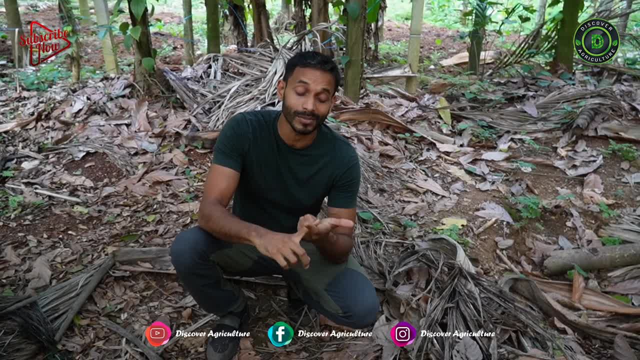 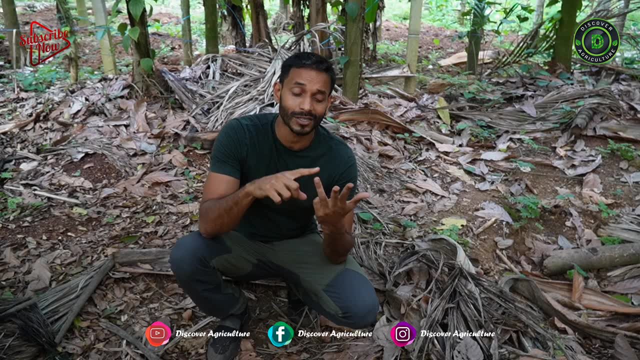 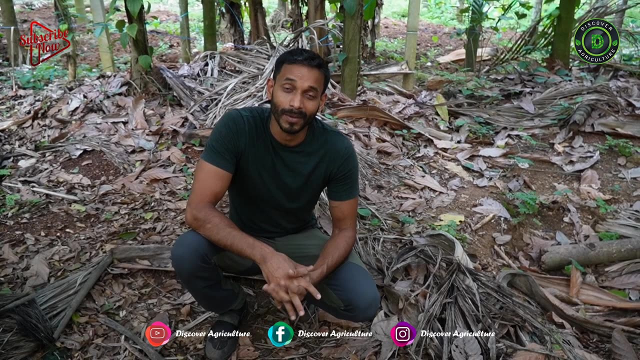 There is a vesicular and vascular mycorrhizal. there is the effective microorganisms. there are consortium of different species of nitrogen fixers, phosphorus solubilizers, potash mobilizers. We will talk about it in the in. this video will take you to our microbiology lab and 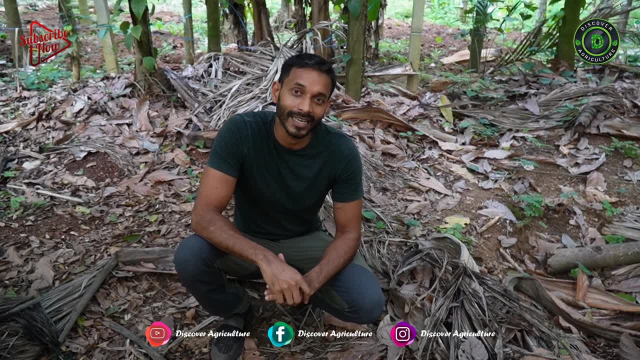 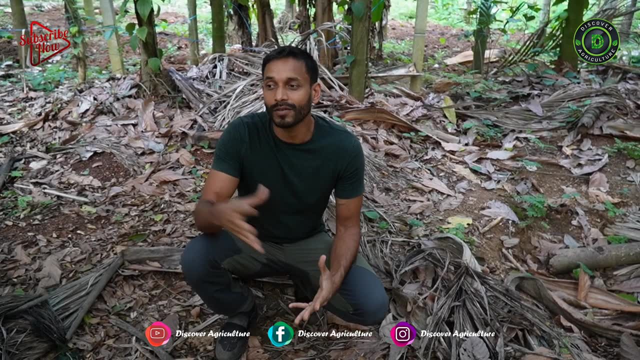 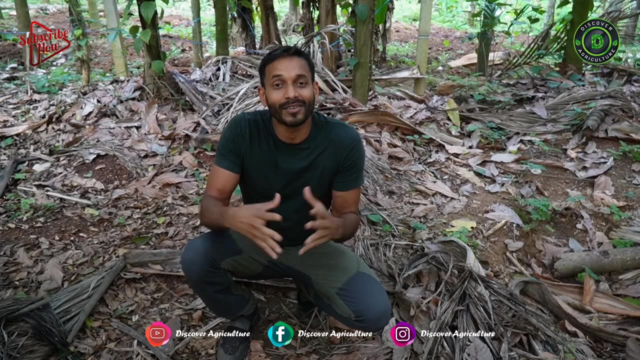 we'll show these different species of microorganisms. These are different species that we have gathered in the last three decades, what we've been using in Varanasi farms, and this is how, one of the primary reasons, along with there are other reasons like a multi crop system and you know the permaculture practices, but one of the main- 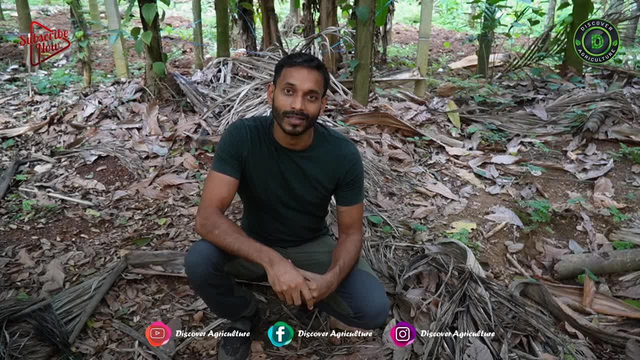 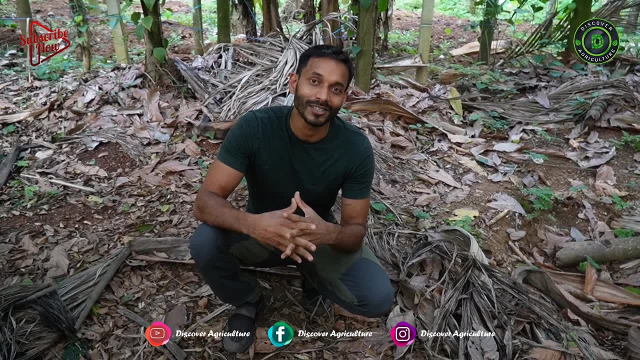 reasons we have this regenerative system at Varanasi farms is because of the presence of beneficial microorganisms, or what we call as biofertilizers and biocontrol agents. Come, let's go to the lab and see what we have here. So let's go to the lab. 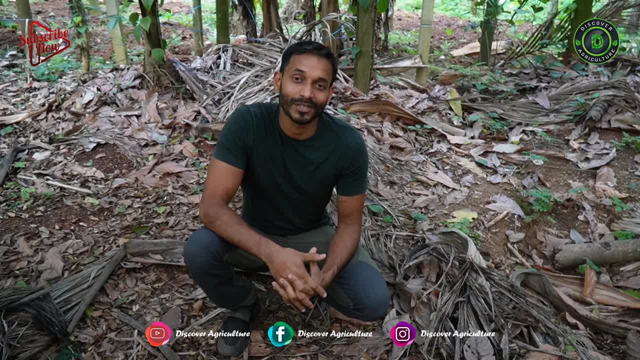 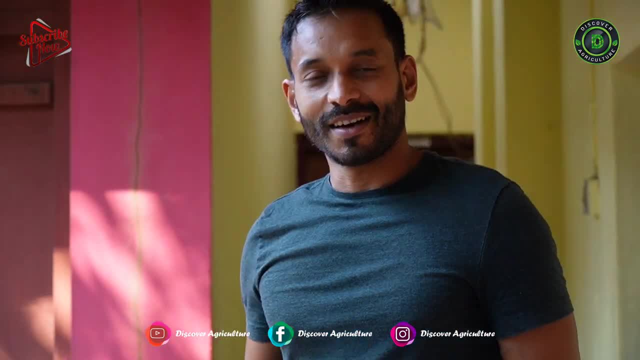 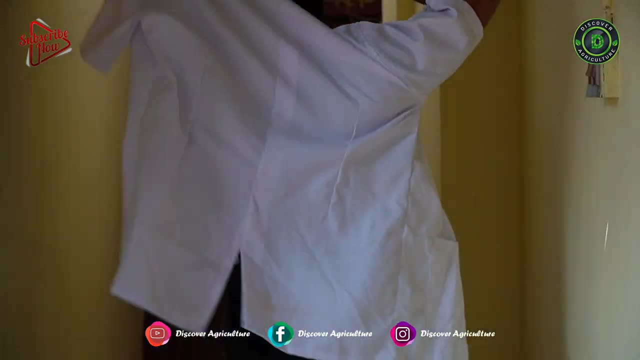 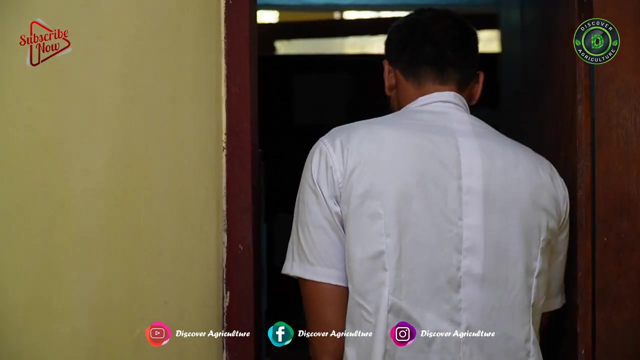 Okay, So let's go to the lab and have a look at these amazing species of microorganisms. which gives us this benefits? Come, let's see our soil microbial mother culture bank. So this is our soil microbial mother culture bank. Okay, So this is our soil microbial mother culture bank. 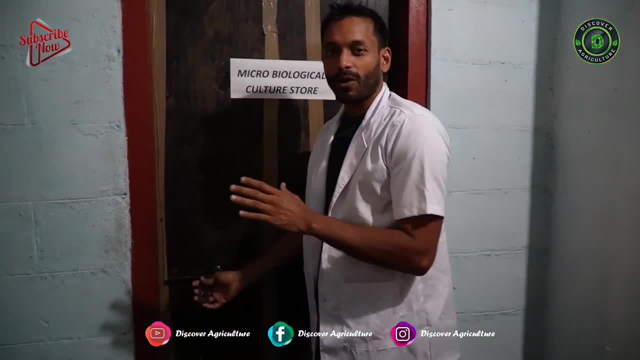 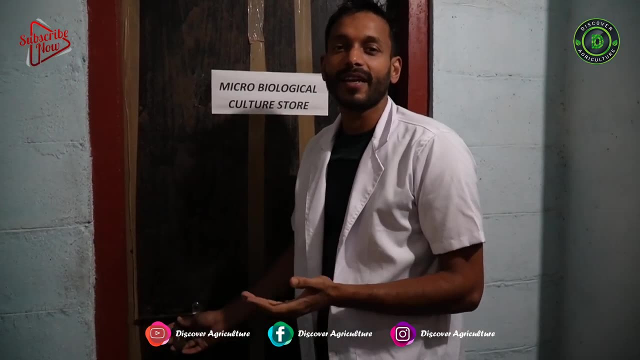 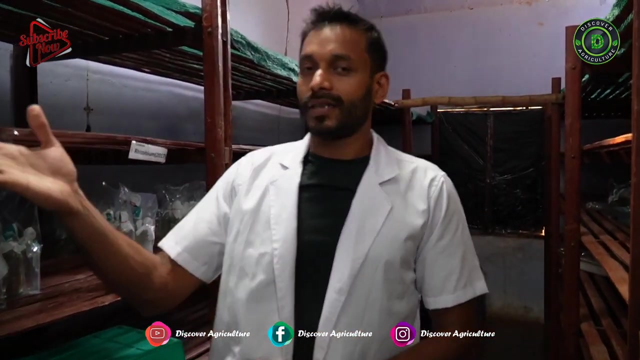 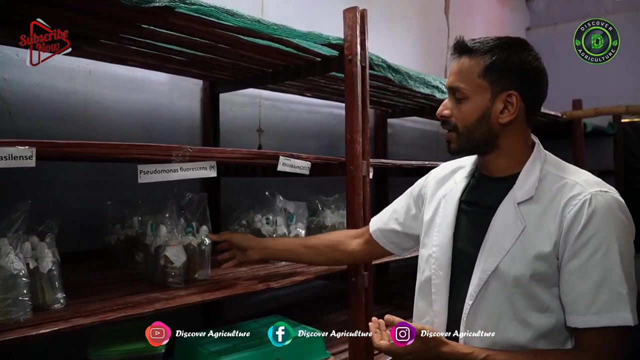 Okay, So this is where we have kept all our different beneficial microbes in Petri dish and we keep sub-culturing it every week and you can see which all we have here. So in here we see Endospirulum, we have Pseudomonas and we have Pseudomonas. 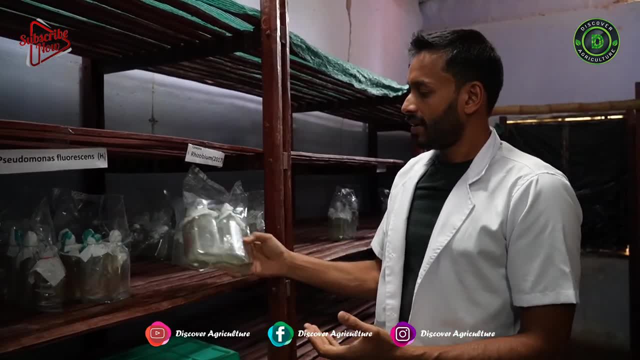 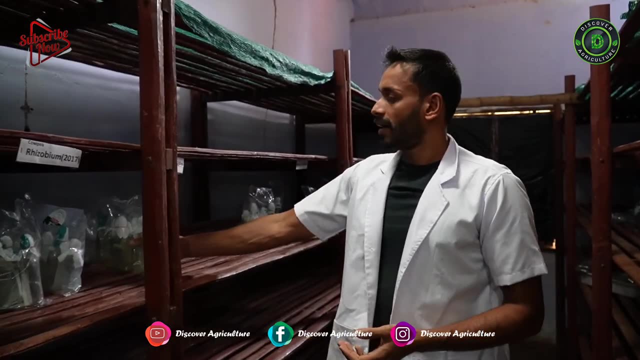 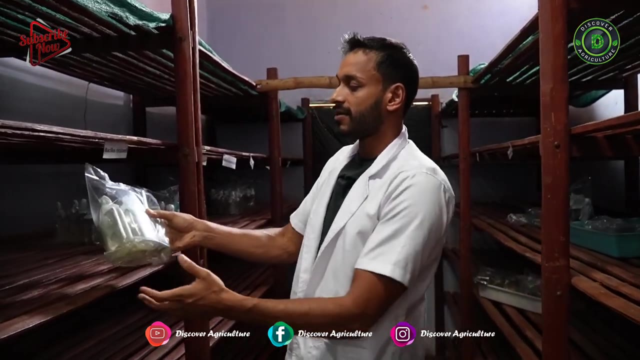 Okay, Okay, Okay, Okay, So this is the placenta. Okay, Okay, So this is Pr. falarum, that involves Somat extraordinaire. Okay, So this is P송an. Okay, Okay. So this is our Phyro filmow, which is Triglyceridum on the 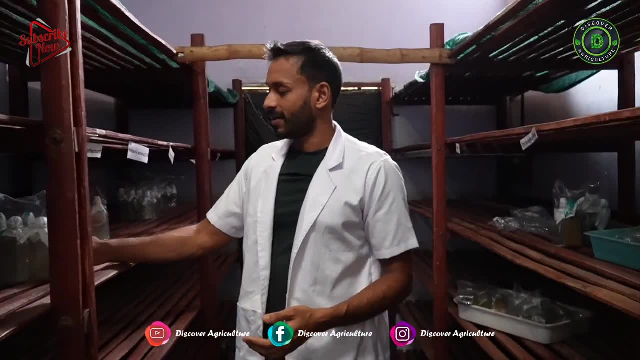 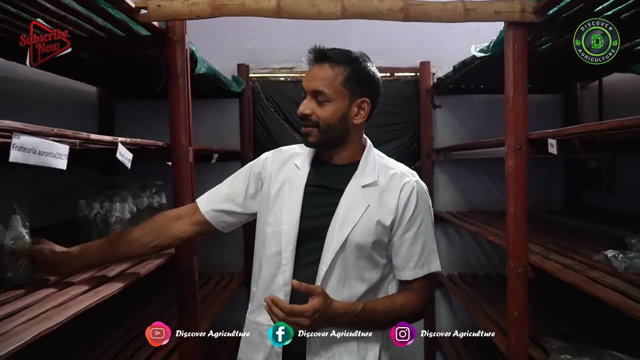 septal, also Mahlossin lactobacillus, by the centre of the body ofrogen. Okay, Okay. So Aminla necessarily has two promise: Virus buenidesis. so the beautiful thing in Patinia is that this is a porcineya brachium, which is a eyelash. 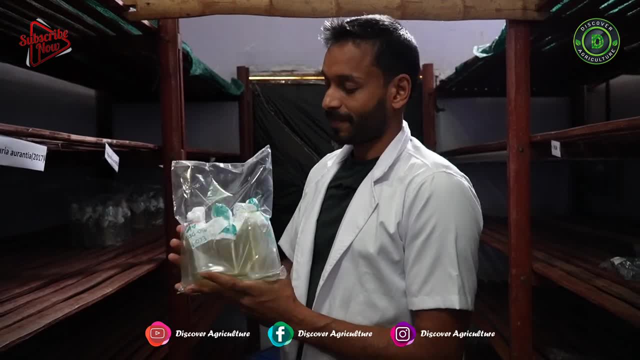 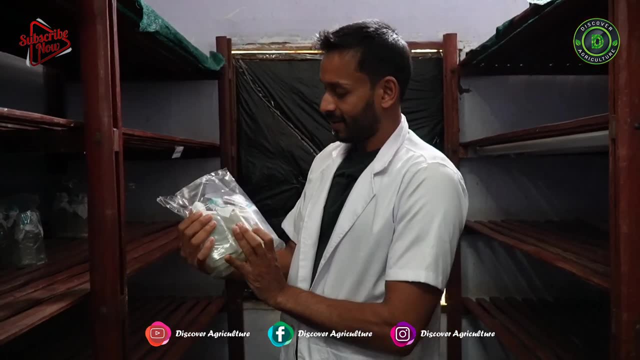 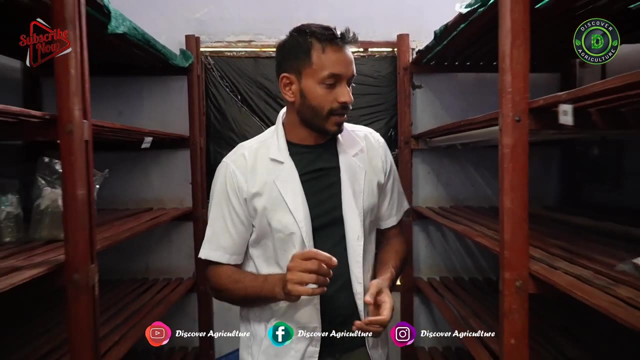 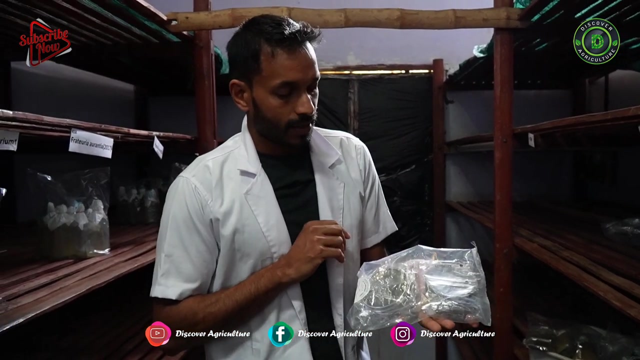 that stands specifically for laxation and vasodwicosis. Okay, attached: mobilizer, a nitrogen fixer, a low-toe backdrop inoculated on the 24th as well, And then we have some common mycelia. this is Trichoderma. you can see this. we recently 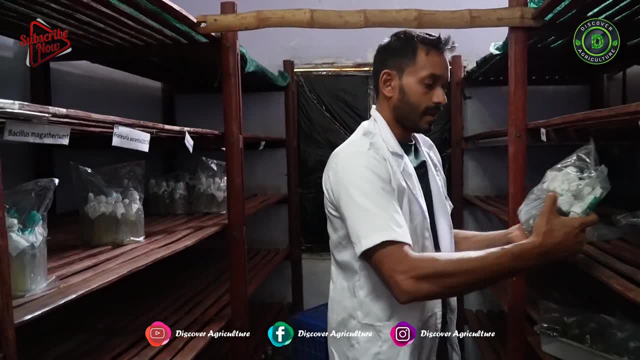 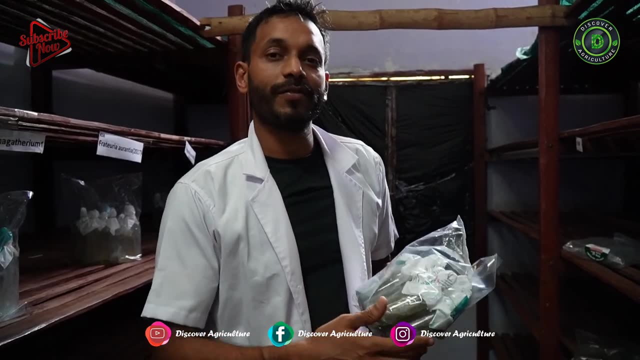 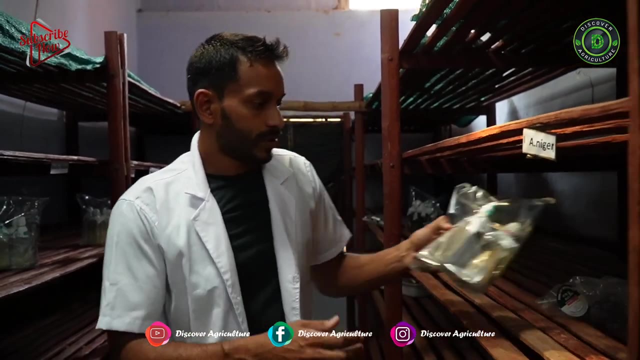 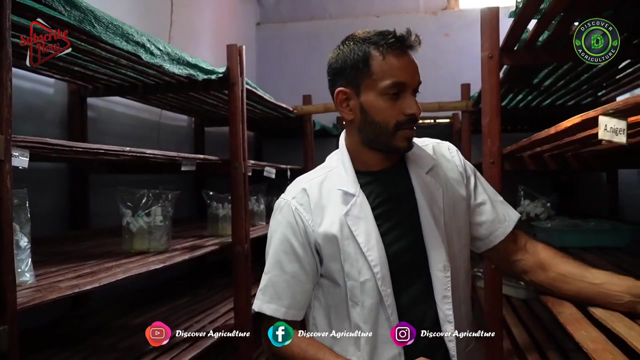 obtained from a university, and this one is something that we have maintained here for the last 15 years. Again, it's been sub-cultured every week, And here we have another fun meal, which is Aspergillus Nigel. Hello friends, 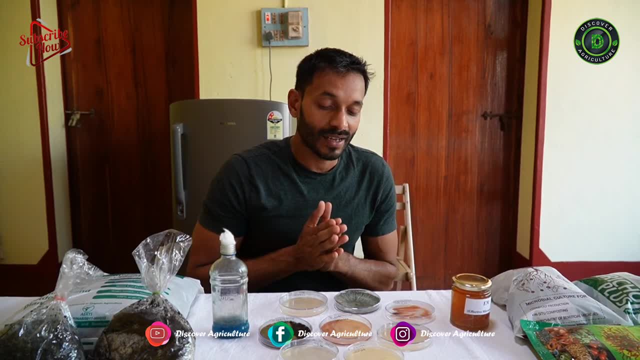 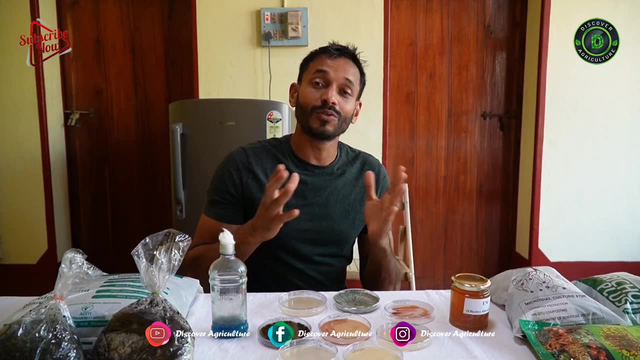 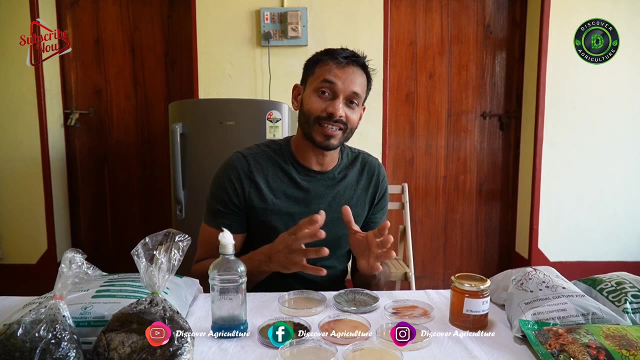 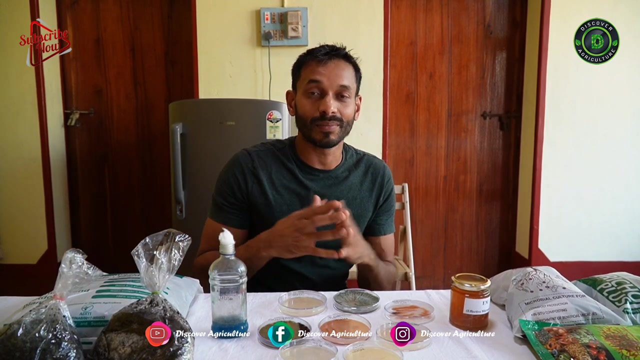 In front of me I have various bio-fertilizers, the soil-borne microorganisms, which are beneficial for the plants. They do two different things: They protect the plants from biotic and abiotic stress. So biotic is basically an infection caused by another microorganism or another living. 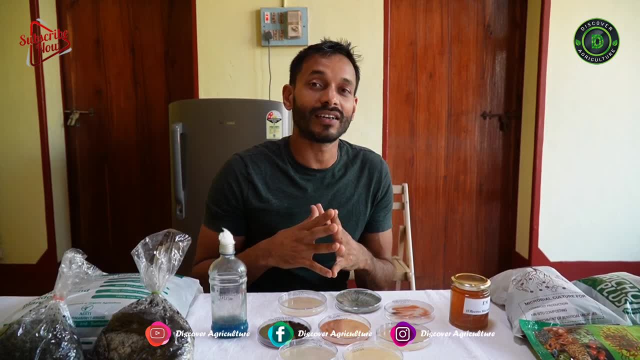 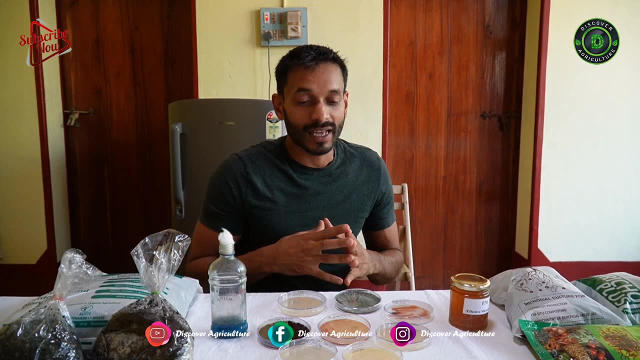 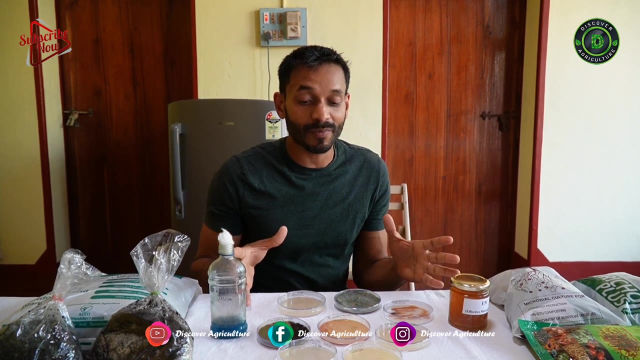 being, as it says, And abiotic stress are the ones which is caused by drought, or higher salinity, or higher pH and all these different situations of the environment. So I'll take you through certain microorganisms which are in front of me, which have been 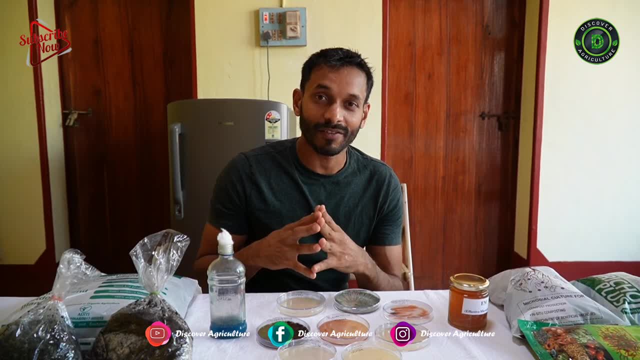 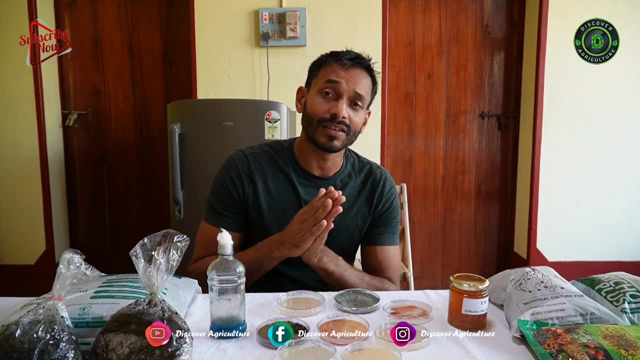 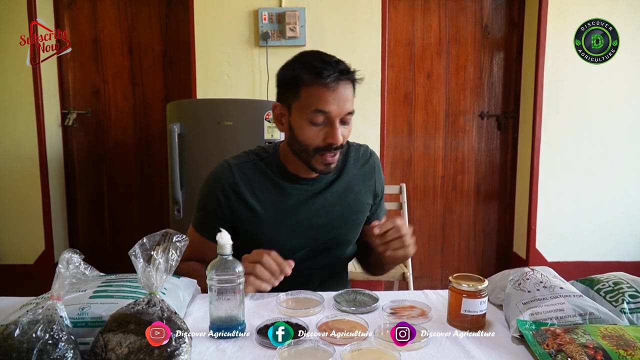 isolated and maintained at Varanasi Development and Research Foundation, And we also produce this through Varanasi Organic Manures and sell it to the farmers so that they can enrich their land with these microbes. So first let's start off with Azetobacter. 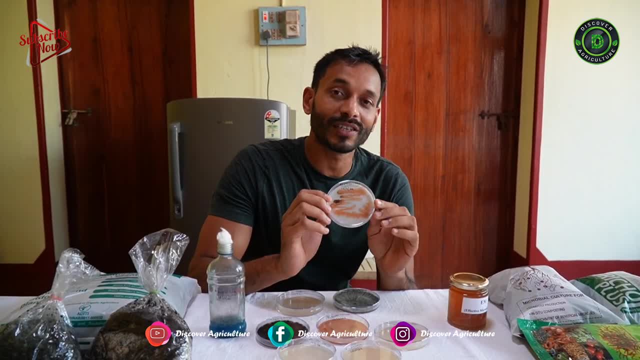 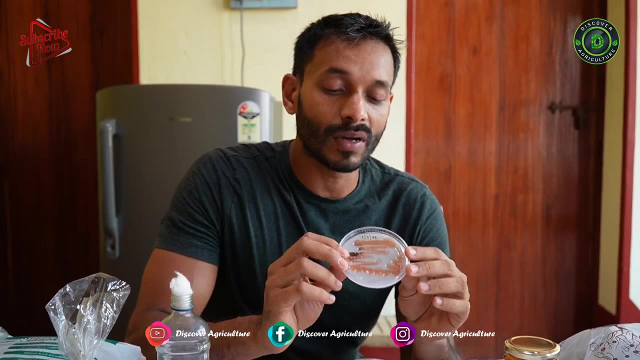 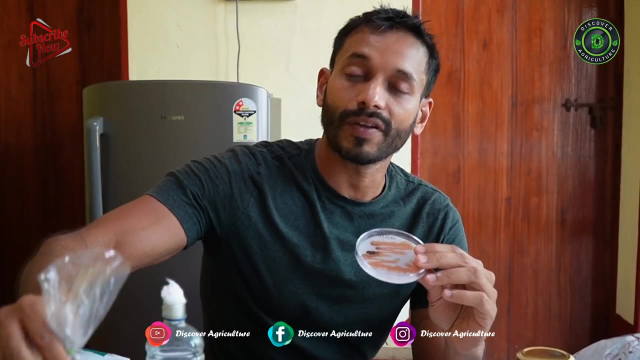 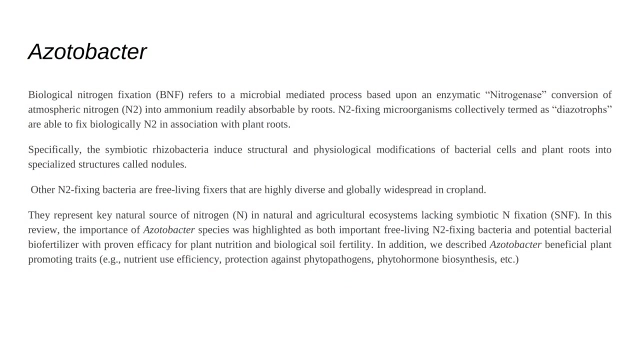 Now, Azetobacter is a plant growth-promoting bacteria. It is found in soil, obviously, So once inoculated into this carrier medium is coffee husk. We spread it across the soil in our plantation. So what it does is it's a nitrogen-fixing bacteria. 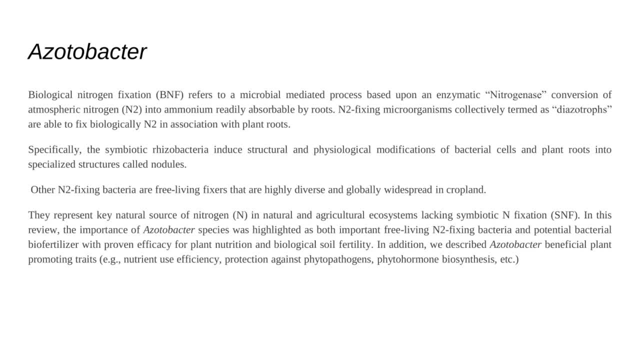 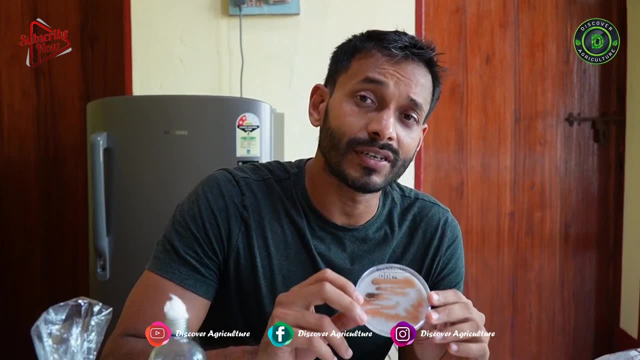 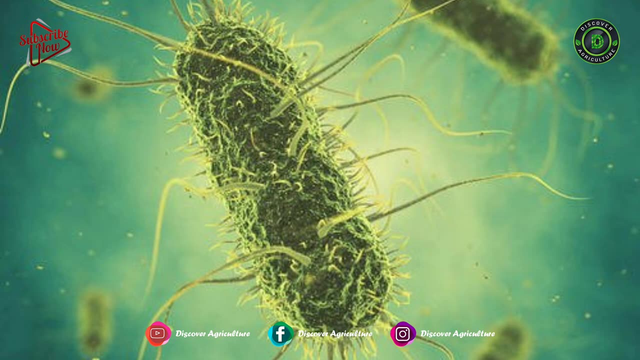 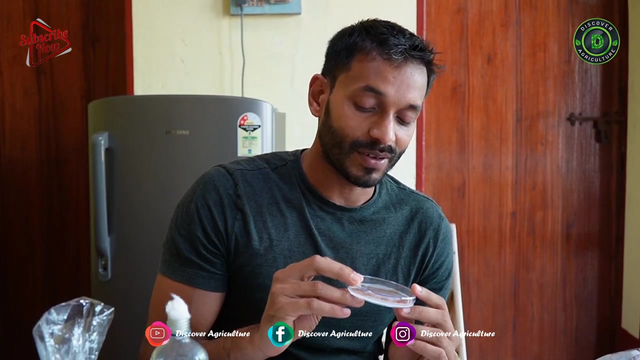 It fixes the atmospheric nitrogen into the soil and makes it bioavailable for the plants, And it also produces certain phytohormones which reduces the effect of biotic and abiotic stress. that's experienced. So there we have. we have Azetobacter. 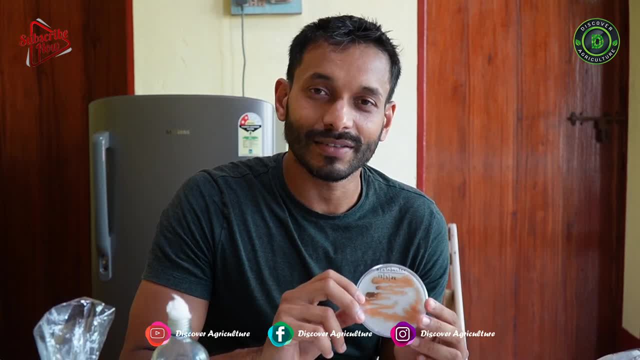 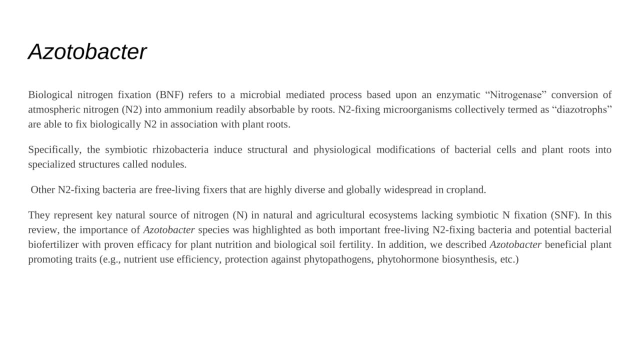 It's also known to produce indoleacetic acid, which is a growth hormone And it's basically overall. the presence of Azetobacter in the soil enhances the plant production, It keeps the pathogens away and also it fixes the atmospheric nitrogen into the soil. 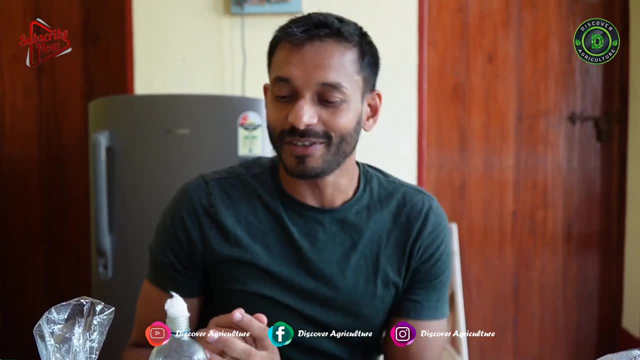 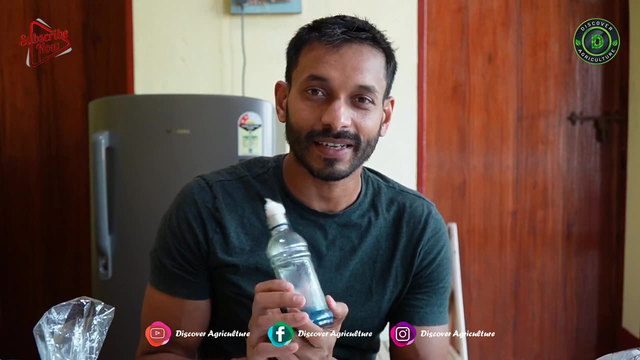 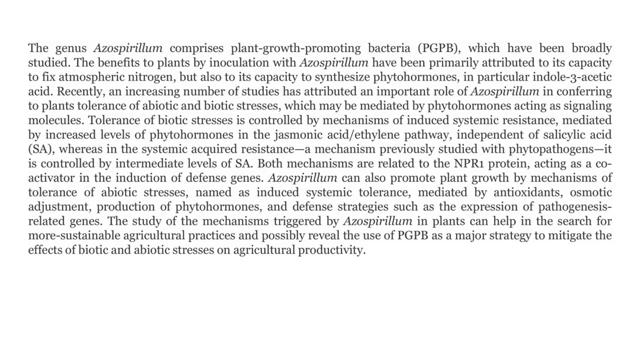 making it bioavailable for the plants. All right, so next up we have this guy. This is Azospirulum. It is also a nitrogen-fixing bacteria. It's a free-living bacteria. It's not, it's a symbiotic. 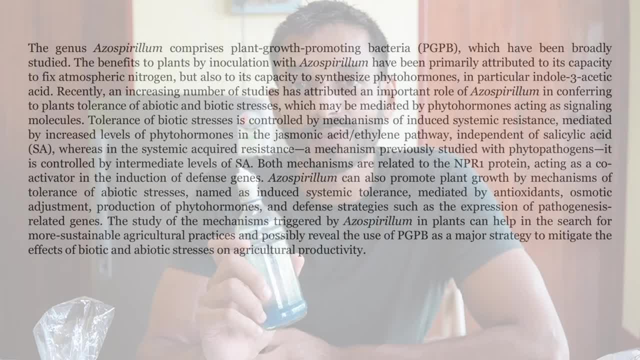 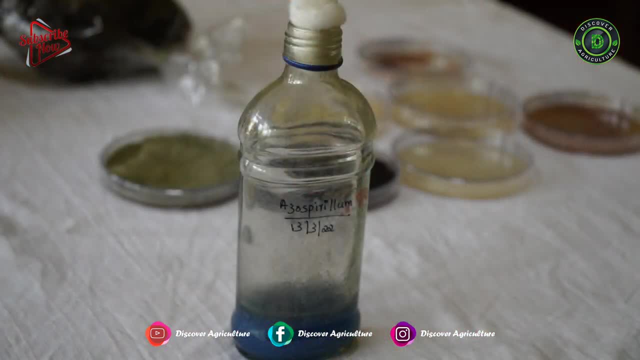 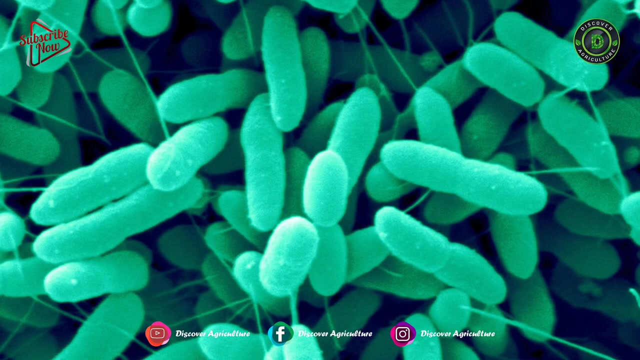 And it also produces phytohormones which kind of fights off the helps the plant fight off abiotic stress such as higher salinity, Variation in pH, drought And also the presence of heavy metals sometimes regulates the plant growth, So this helps the plants fend it off. 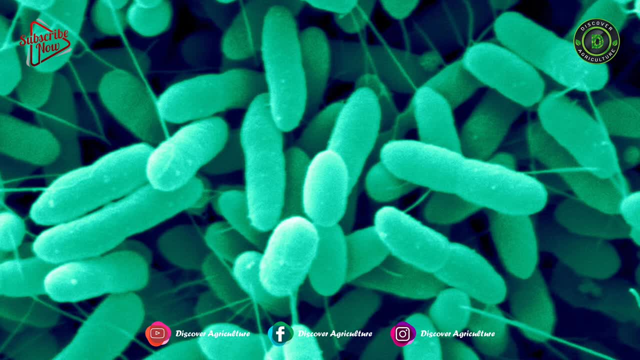 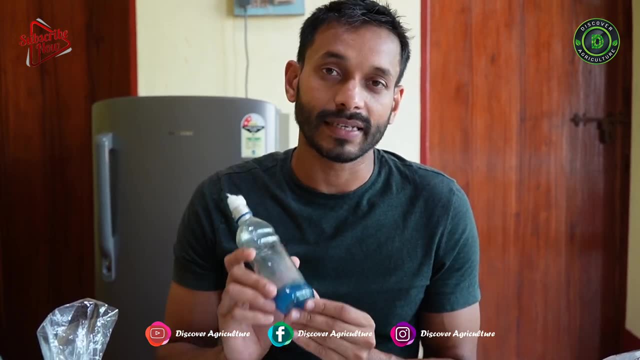 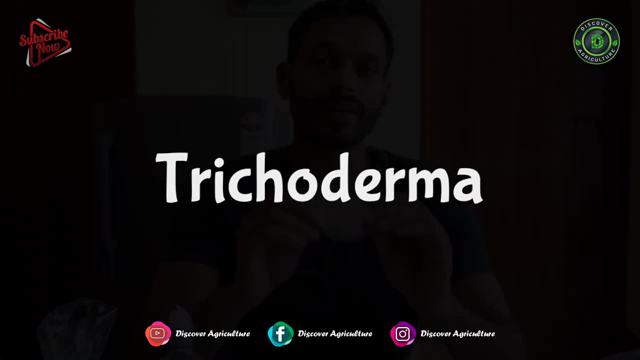 And also it's: it produces growth, growth hormones, So helping the plants to grow better. So that is Azospirulum, It is a bacterium as well, And then we have: okay, let's go into, okay, let's go into Trichoderma here. 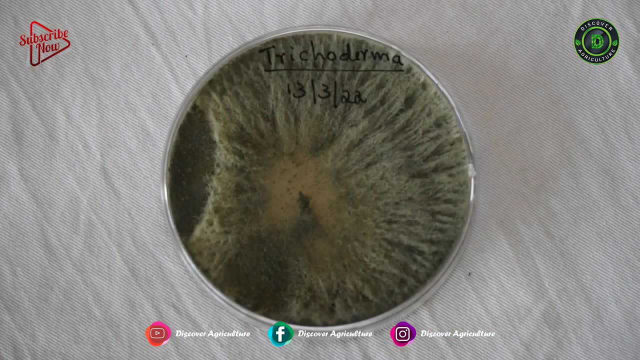 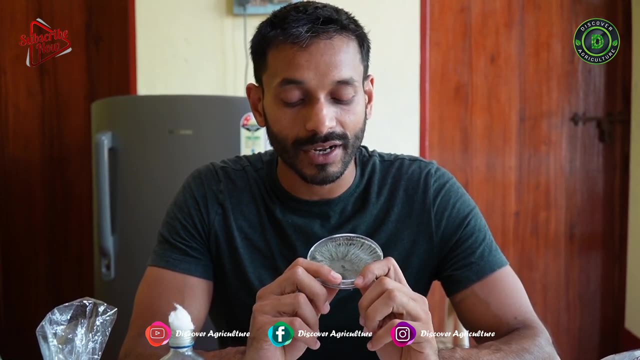 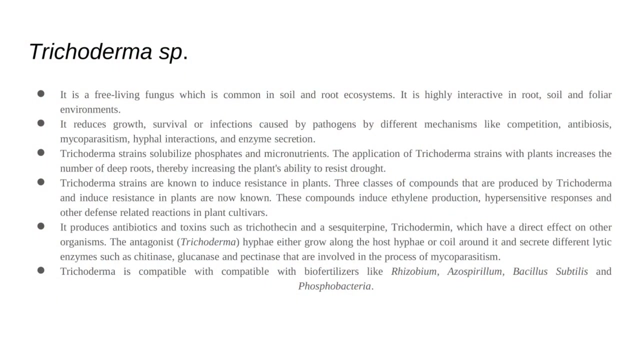 Trichoderma, one of our favorite. This is a fungus And it's also a biocontrol agent, So when there is Trichoderma growing in your farm, it keeps away the pests, like the pathogens such as Fusarium and Phytophthora. 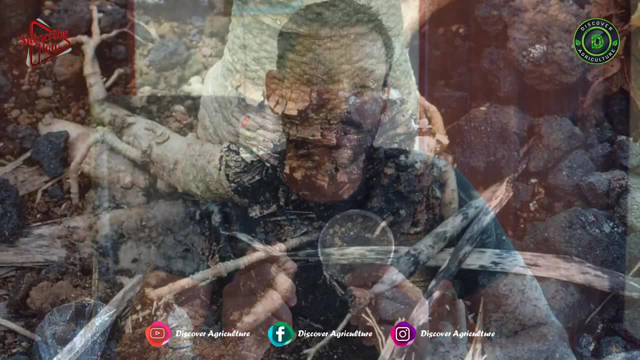 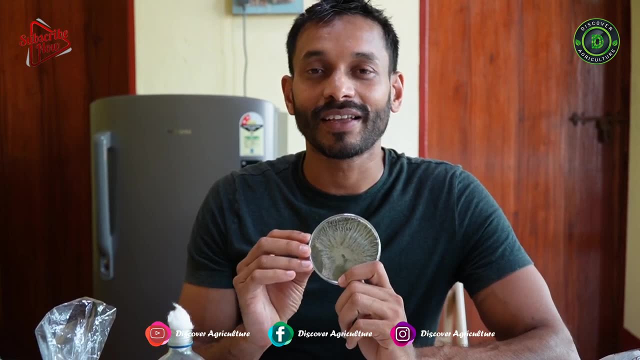 So we know that Fusarium and Phytophthora causes the root rot and the wilting end, the root rot, The root rot disease respectively, And this is a natural enemy of Phytophthora and Fusarium. So in the presence of Trichoderma they do not. 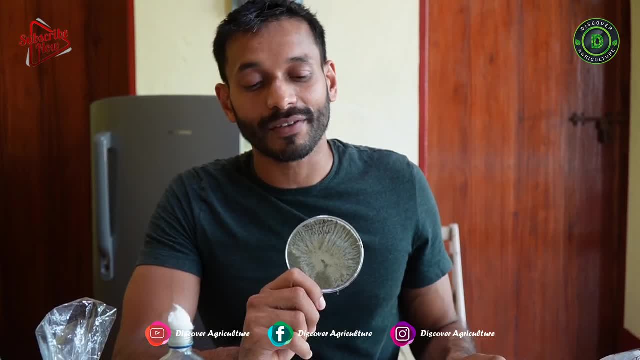 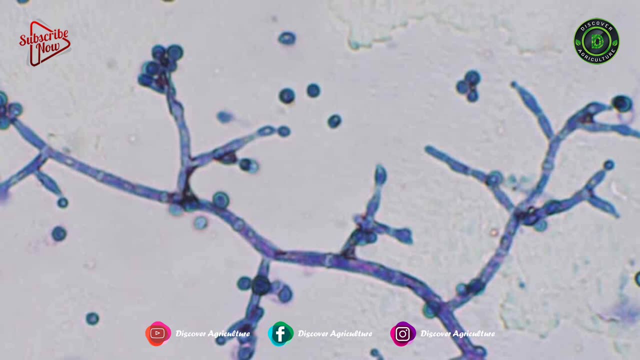 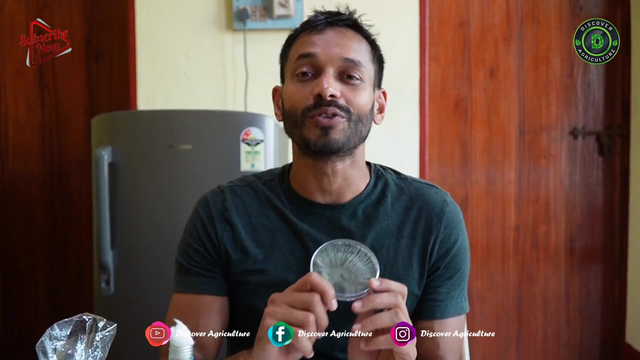 they don't thrive. The pathogens do not thrive in your farm. Thus, this protects your plants from these diseases. At the same time, it's known to produce indole acetic acid, which is a phytohormone which increases the shoot growth. 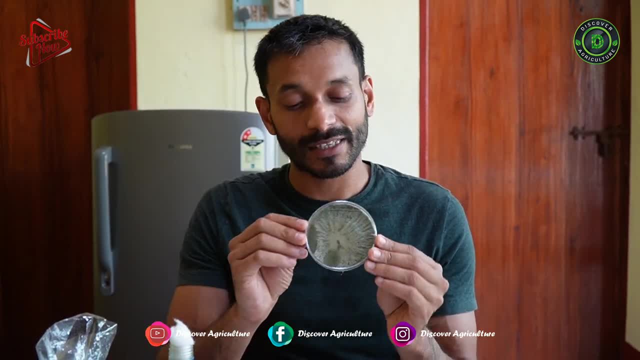 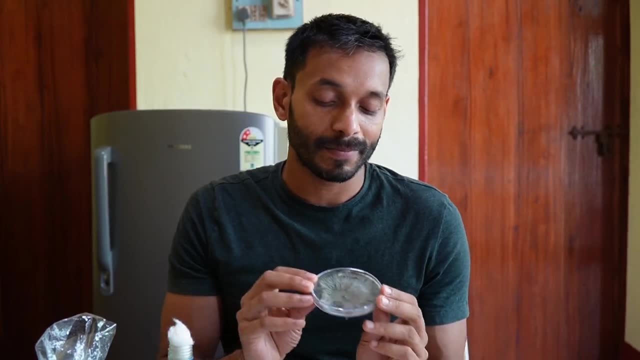 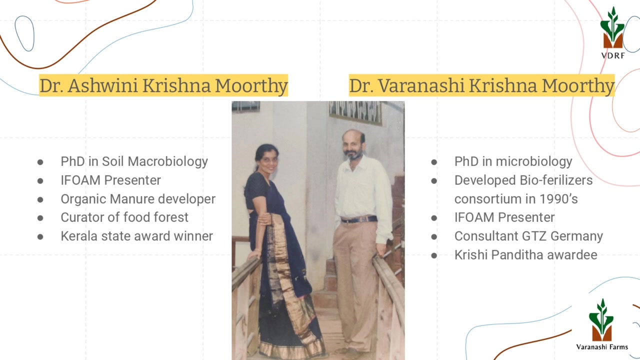 So that's Trichoderma. You can see the colonies and spreadings over here. It's coming beautifully. So at Varanasi Research Foundation, my father, Dr Varanasi Krishnamurthy, found this accidentally. It's the first biofertilizer that we started in here. 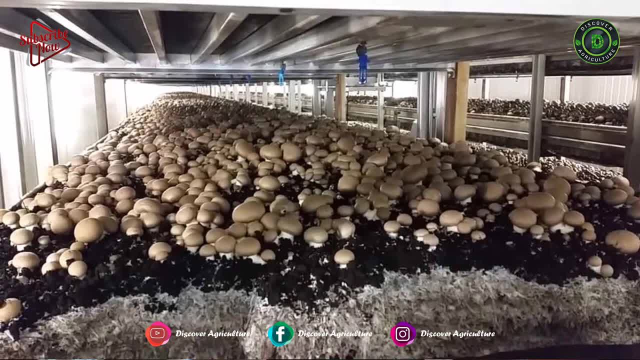 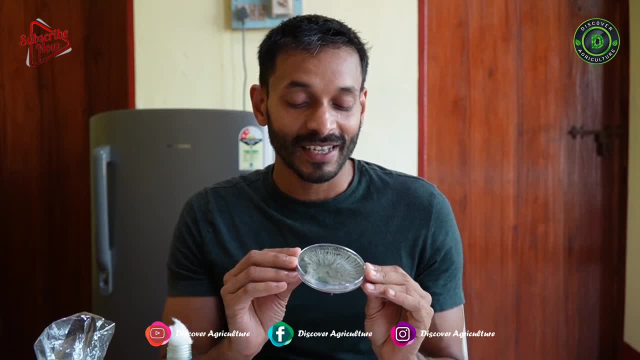 It came in as a pathogen for mushrooms And when he was studying what it was, he read different articles, science articles, and found out that it's a biofertilizer. This is how our story into biofertilizers started three decades ago. 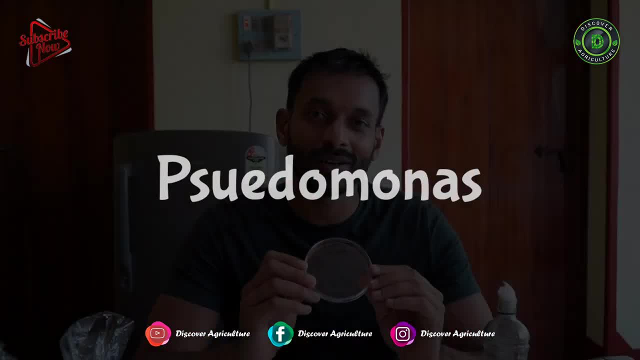 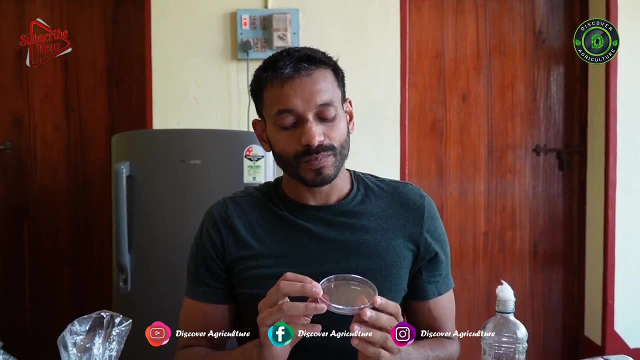 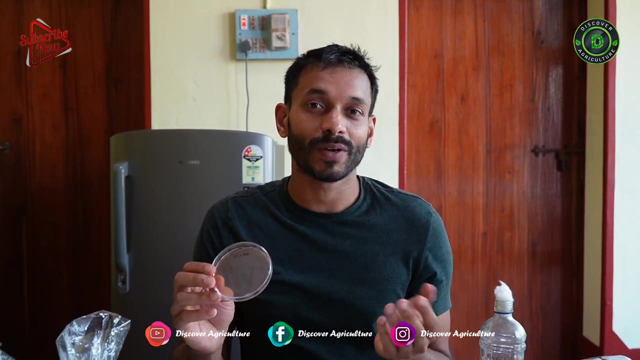 Trichoderma. So next up is Cerumenase, which is in my hand. This is a quite famous biofertilizer. What Cerumenase does is it kind of dominates in the rhizosphere and it keeps the pathogens away. 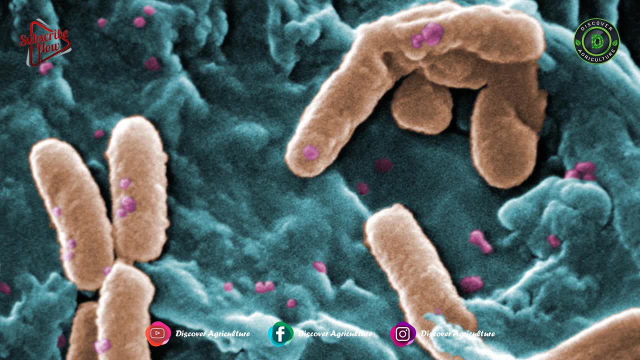 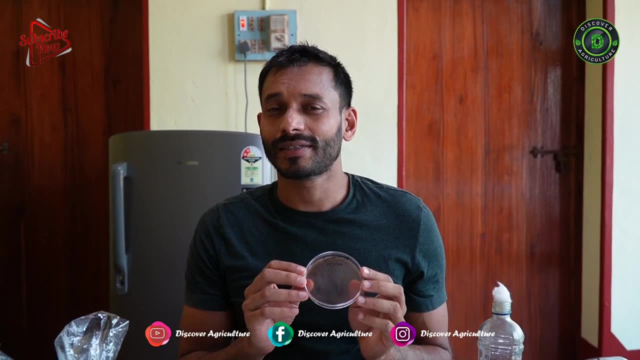 It is a phosphorus solubilizer. It makes the phosphorus more bioavailable for the plants. It also produces phytohormones, such as auxins and gibberellins, which are both shoot and root promoters, So it acts as a growth promoter. 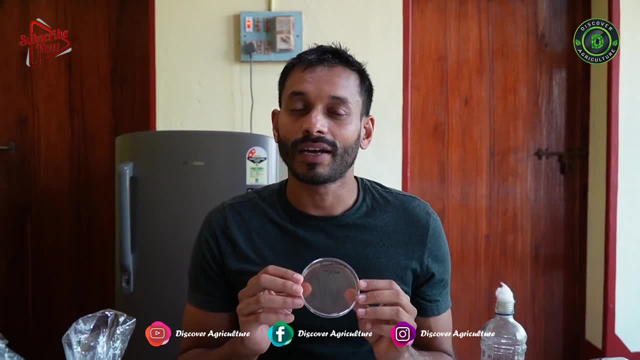 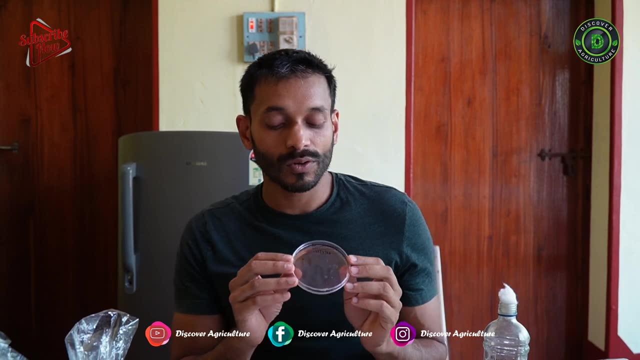 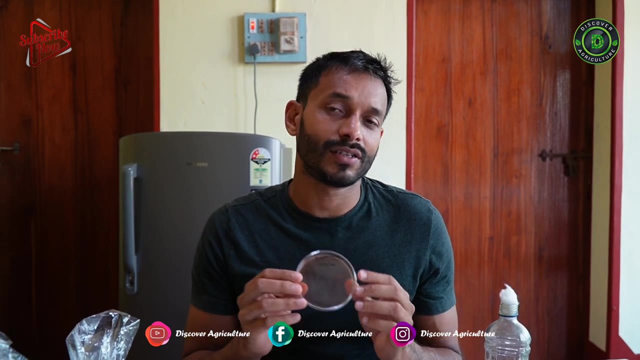 And it also produces secondary metabolites, which keeps the pathogens away and keeps the plant healthy. So that is Cerumenase, And Cerumenase grows well, along with certain other biofertilizers such as Aspergillus and Trichoderma. 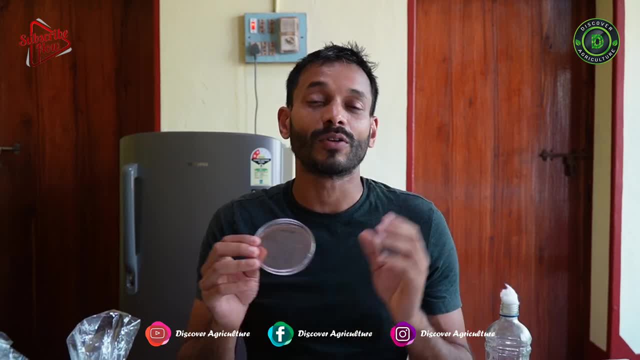 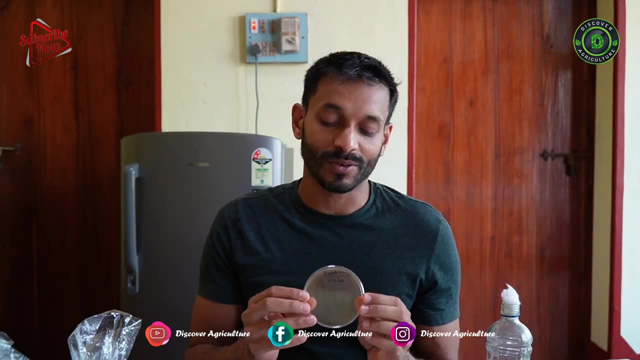 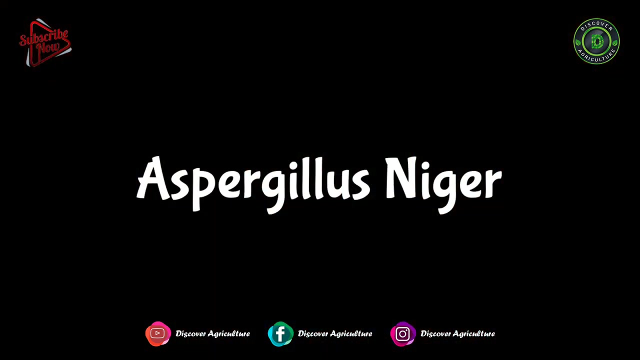 And some bacterias as well. So they all group up together and give that support required by the plants. These guys support it. So there you go, Cerumenase, And then next let's have Aspergillus nigellus. 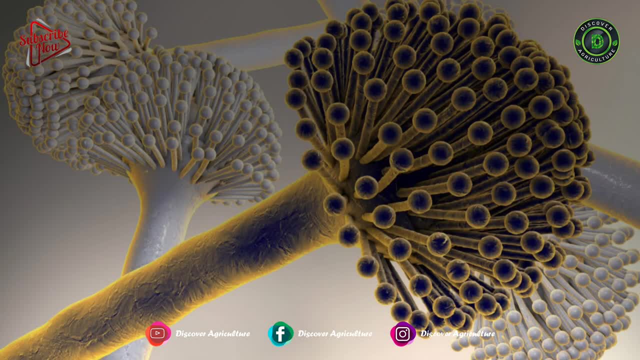 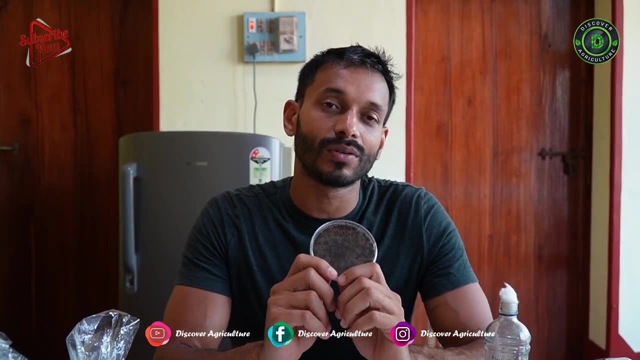 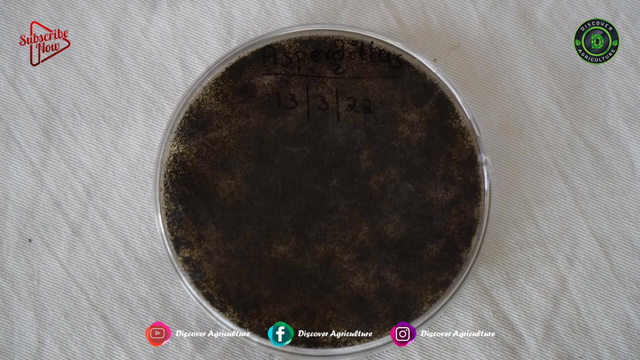 It's a fungi, And Aspergillus also produces phytohormones. It supports the plant growth. It is also a phosphorus solubilizer, just like Cerumenase, And all these fungi work hand-to-hand together and help the plants grow faster. 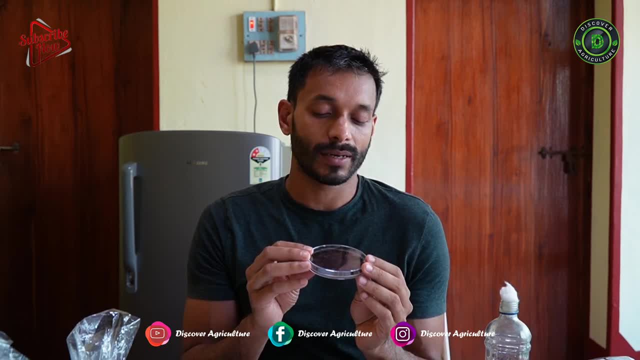 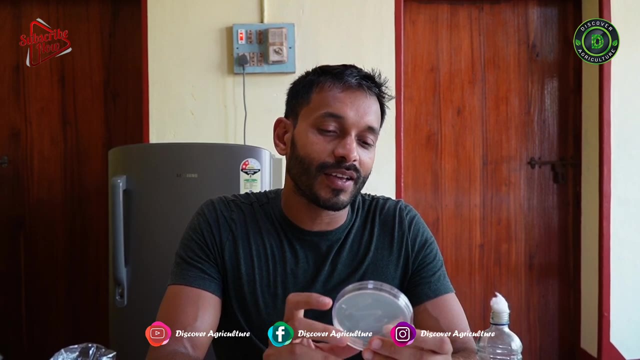 So Aspergillus nigellus is also the one I have in my hand. It's a great biofertilizer which grows in the rhizosphere and supports the plant growth Alright. so next up, we have Bacterium, And this is Bacillus megatherium. 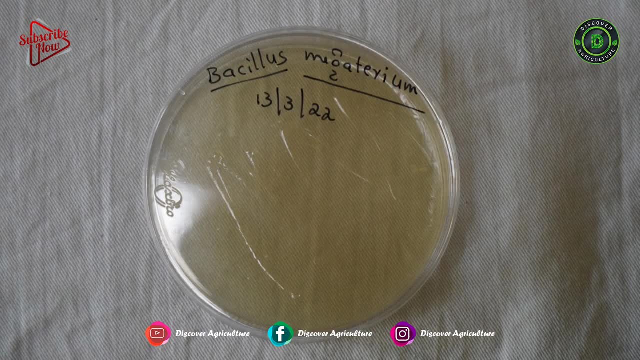 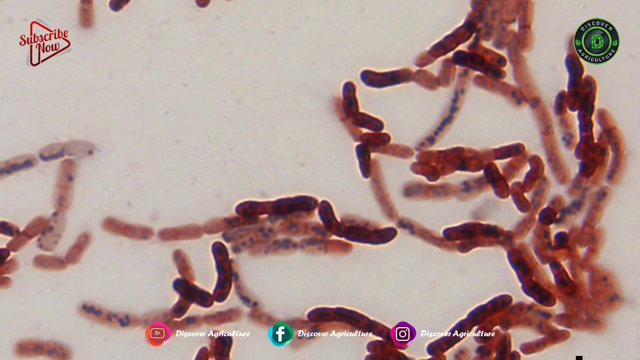 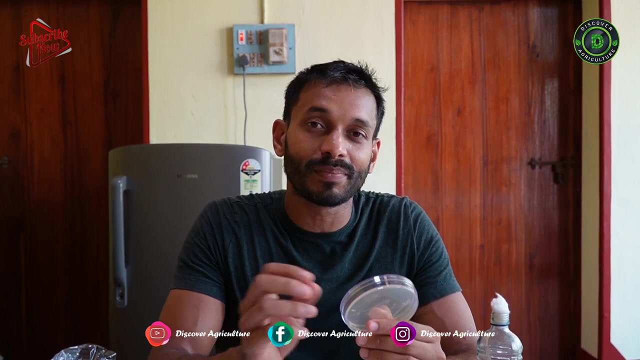 Bacillus megatherium is a gram-positive rod-shaped endospore-forming bacteria. It's an effective soil inoculant, So once it's in the soil it multiplies rapidly And it doesn't allow the other pathogenic bacteria or fungi to come near it. 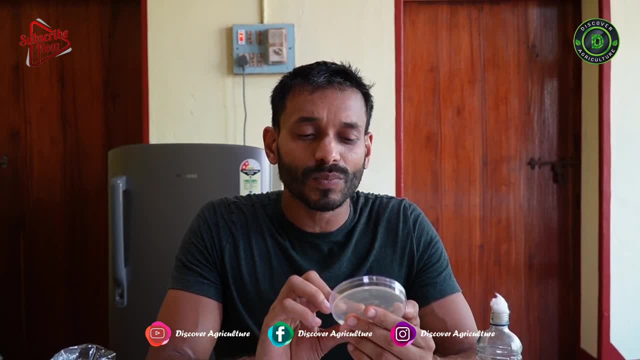 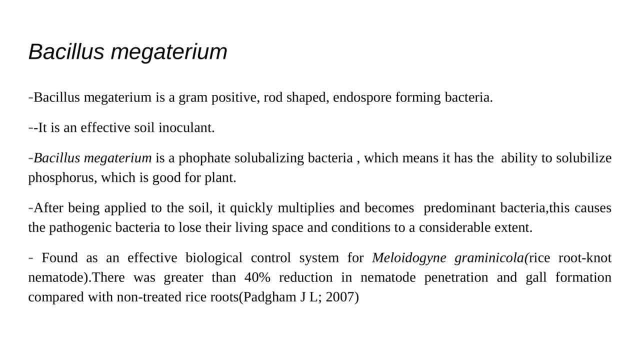 So that way it is a great biocontrol agent. It's also a phosphorus mobilizing- Sorry. It's a phosphorus mobilizing microorganisms, which allows the plant to get the phosphorus readily. Bacillus megatherium is also found as an effective biological control system. 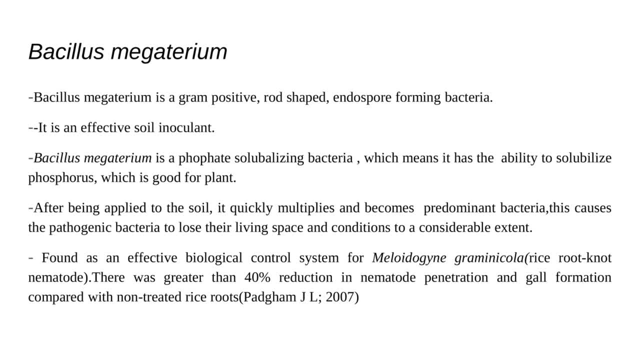 for the rice root, not nematode. So there was a greater than 40% reduction in nematode in the presence of Bacillus megatherium. So it's also a fantastic biocontrol agent and also a biofertilizer. 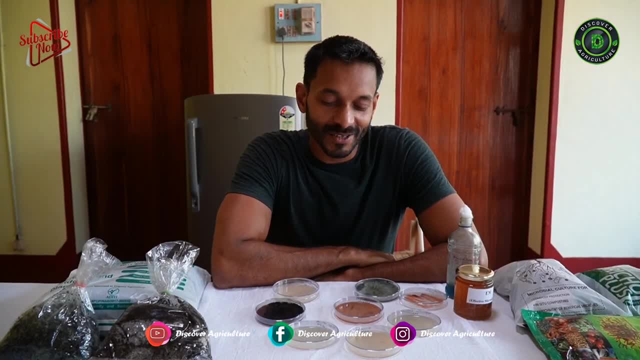 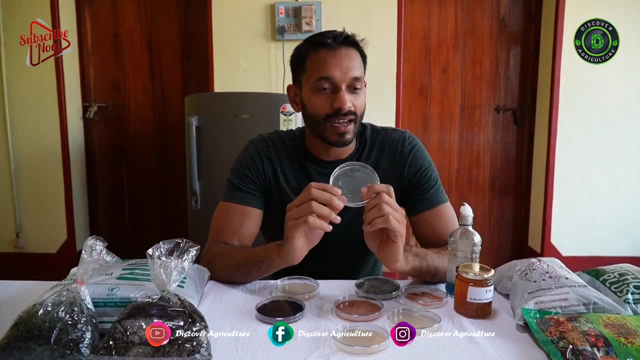 So that's Bacillus megatherium. Okay, so next up, we have in our collection Bacillus subtilis. Now, Bacillus subtilis is a gram-positive endospore-forming bacteria which is also a biocontrol agent. 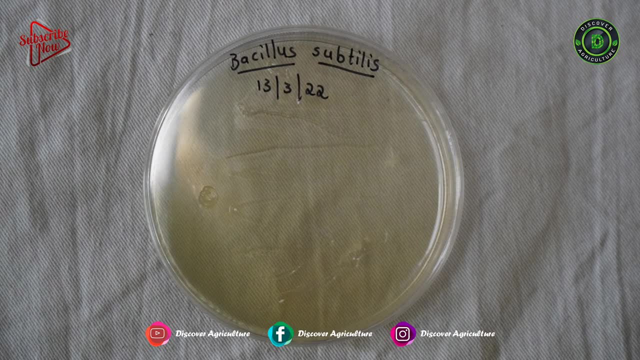 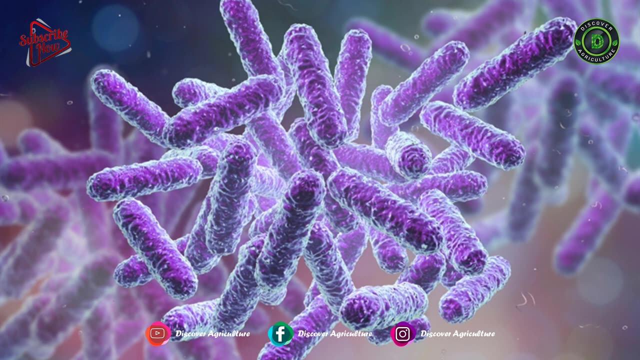 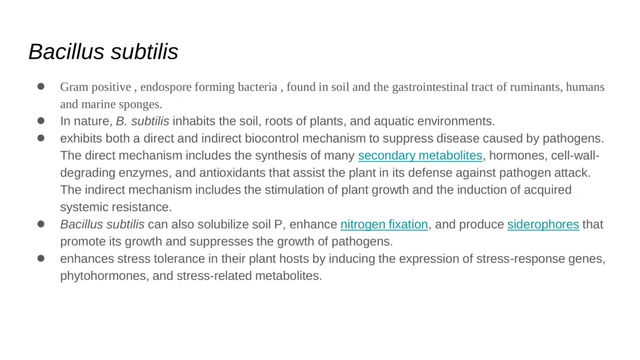 It's found in the soil, It's found in the root zones, It's found in aquatic environments and also just present in the soil. So Bacillus subtilis exhibits both direct and indirect biocontrol mechanism to suppress the disease caused by pathogens. 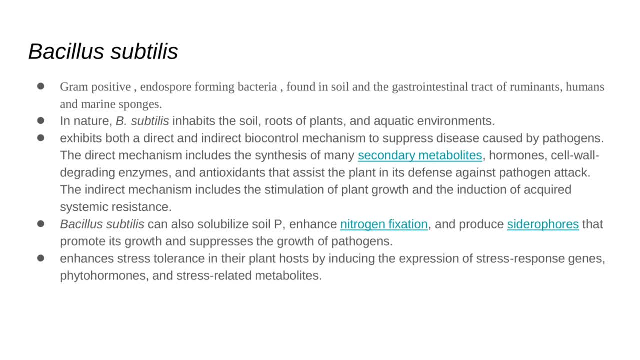 So the direct mechanism is basically it produces secondary metabolites such as hormones, cell wall-degenerating enzymes, antioxidants, which assist the plants to attack these pathogens and kill them off, fend them off. And the indirect mechanism includes the stimulation of plant growth and induction plant growth hormones. 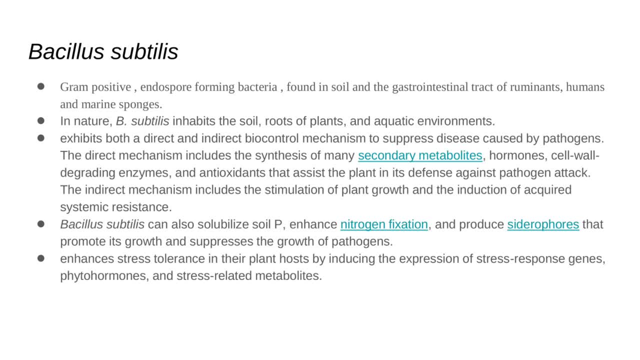 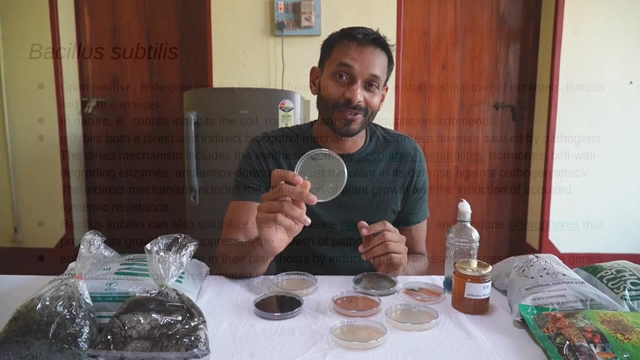 and also induction of acquired systemic resistance. So year by year. in the presence of Bacillus subtilis, the plant identifies the pathogens and produces certain mechanism it needs to restrain these pathogens and grow happily. So that's Bacillus subtilis. Along with it, it is also a nitrogen fixator. 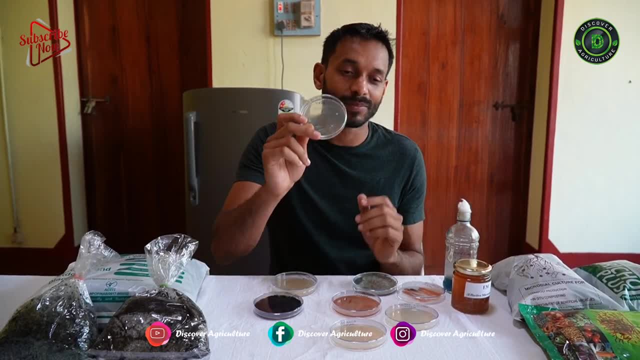 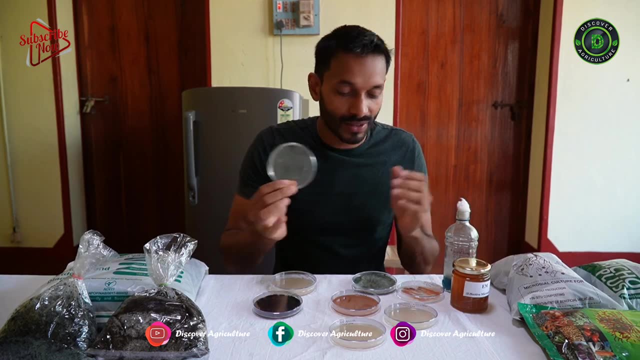 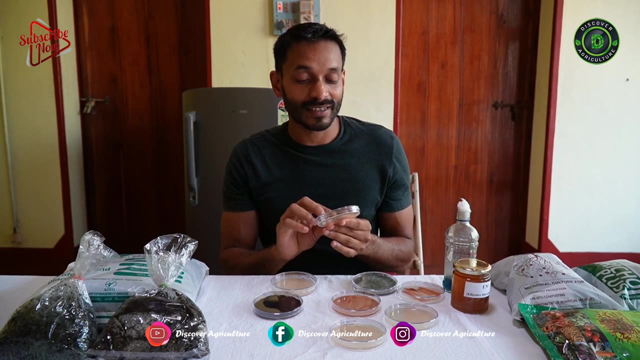 So it's a very interesting bacteria and also helps in phosphorus solubilization, So multiple benefits. And it also comes up in a consortium of other, these beautiful microbes which assist the plants all together. So there you go. The universe has created Bacillus subtilis with a certain thinking. 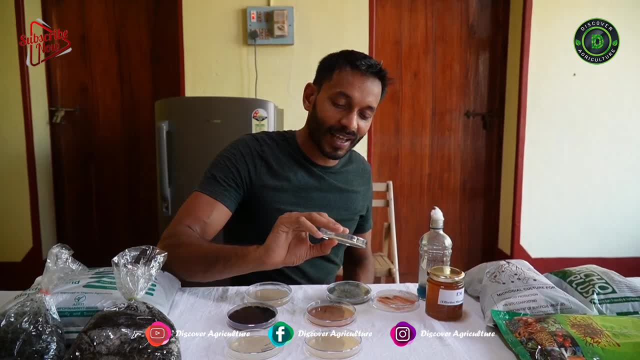 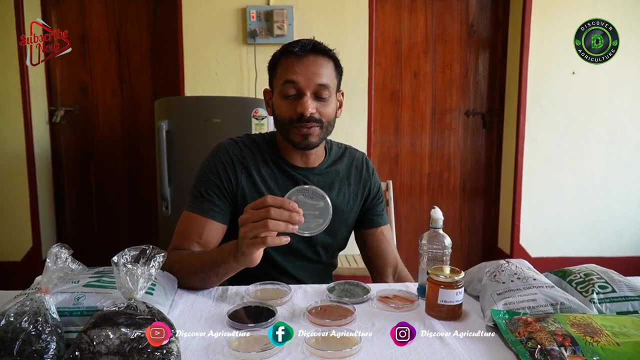 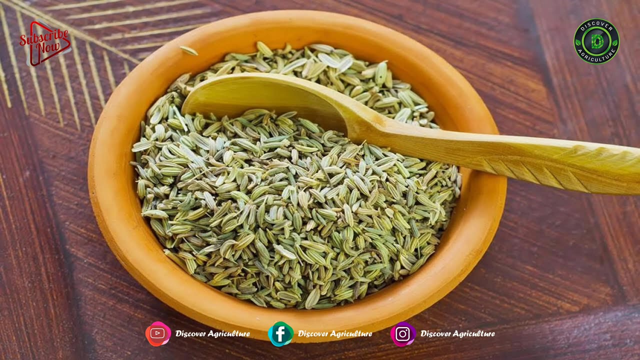 And I think it's beautiful, All right. So next up we have Bacillus circulans, And recently they did a study in Kanpur where they inoculated Bacillus circulans into the fennel producing fields And apparently the color and the taste of fennel seed was much brighter. 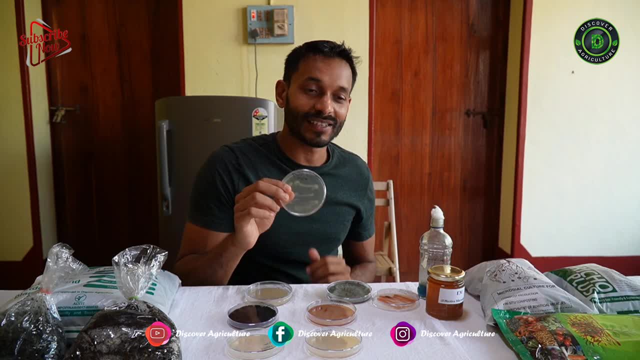 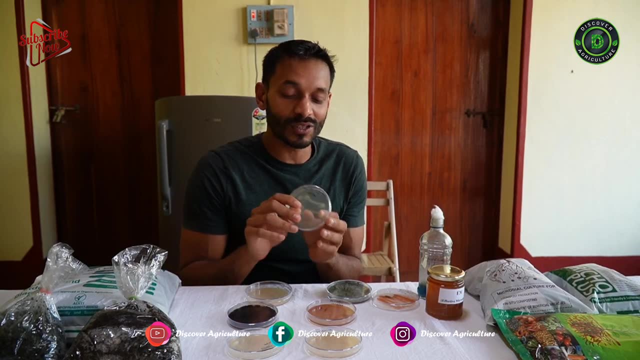 and tasty crunchier after using Bacillus circulans. Bacillus circulans goes really well with vesicular and vascular mycorrhizae And in the root zones it helps solubilizing of potash and makes it more bioavailable for the plants. 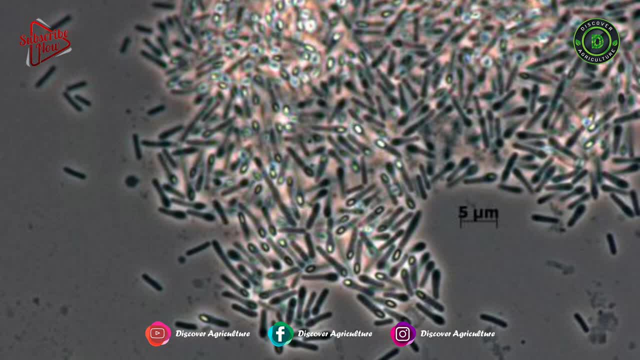 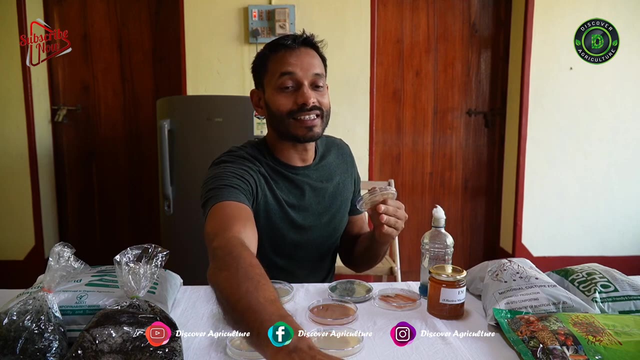 The problem with the phosphorus is it combines with iron, zinc, magnesium and it is not bioavailable for the plants. Even though phosphorus is present in the soil, when you do the soil testing, it just comes up as like a phosphorus deficient. 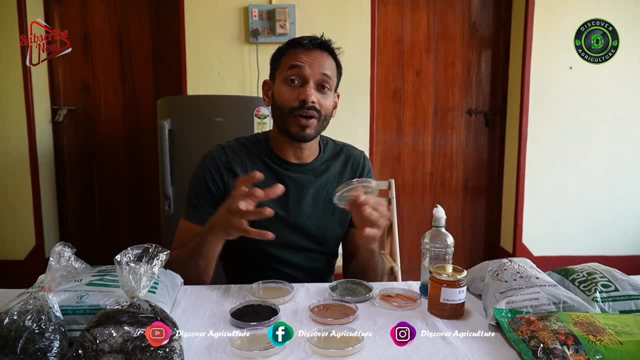 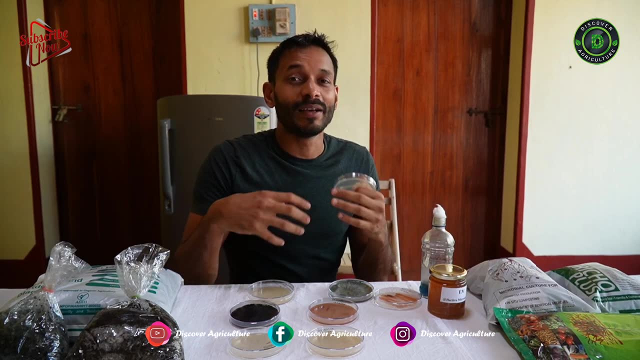 That's not because phosphorus is not present there. It is not bioavailable there, It just simply combines with other cations and forms a complex, Making it not bioavailable for the plants. That's why we need phosphorus, solubilizing bacteria and fungi. 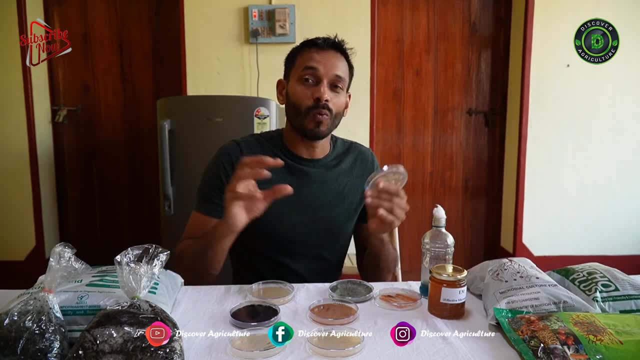 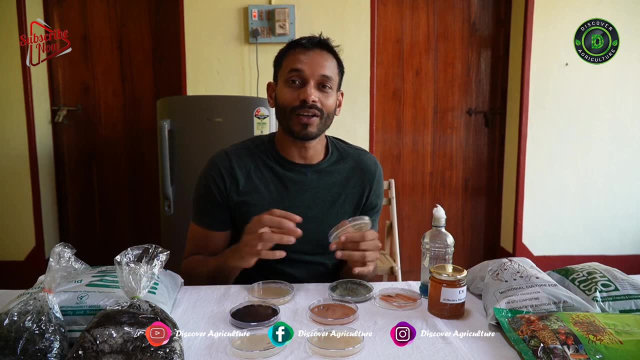 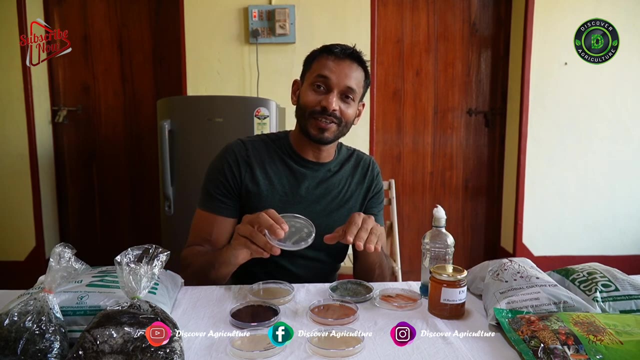 Not just the circulans, all the other I mentioned earlier as well- Which goes and separates these phosphorus from the cations and makes it more bioavailable for the plants. So if your place is phosphorus deficient, that doesn't mean that you should put more phosphorus into it. 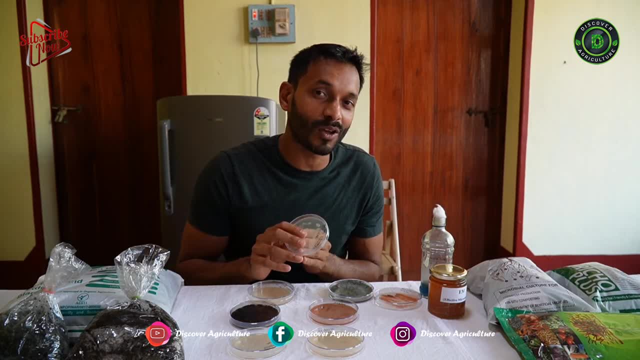 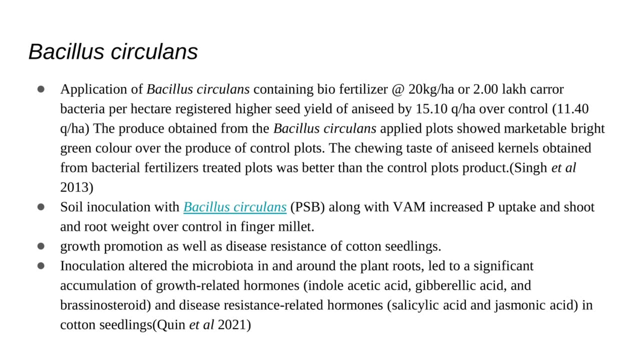 You should probably inoculate more phosphorus solubilizing bacteria or fungi, Which is going to help you improve your phosphorus or the nutrient availability for the plants. So, along with this, it also has plant growth promoting hormones- phyrohormones. 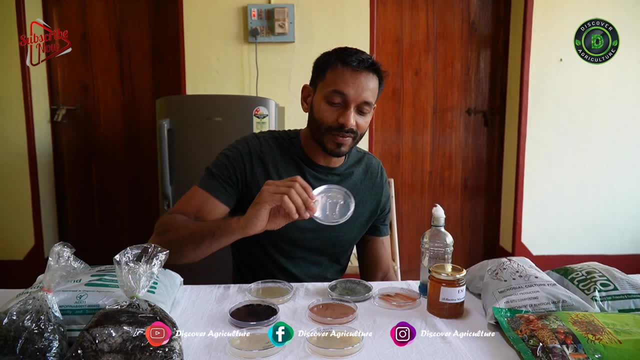 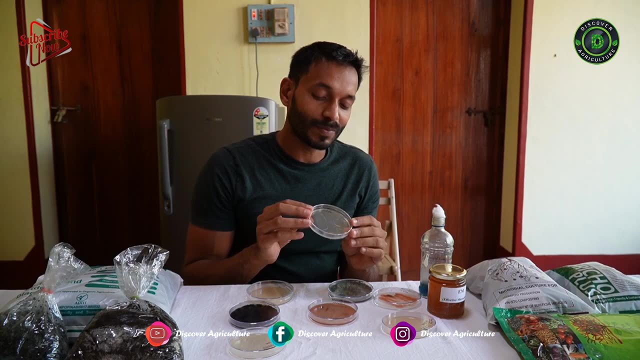 So overall, bacillus circulans is also a fantastic biofertilizer. So next up is the fraction Fracturea. Fracturea is the only potash mobilizing bacteria that we have. It is known to increase the efficiency of photosynthesis. 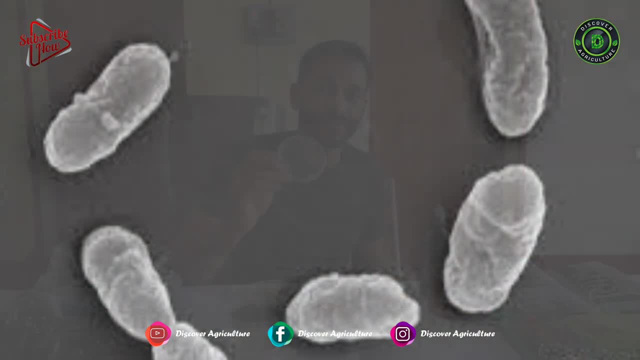 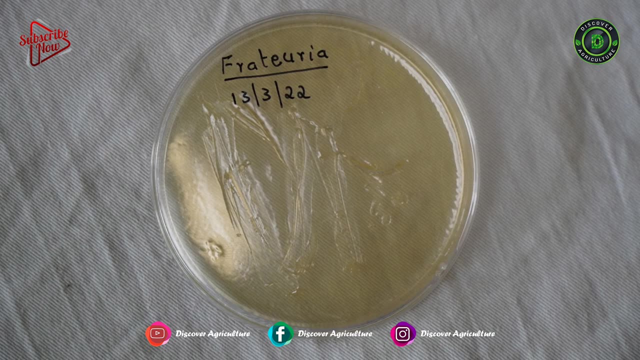 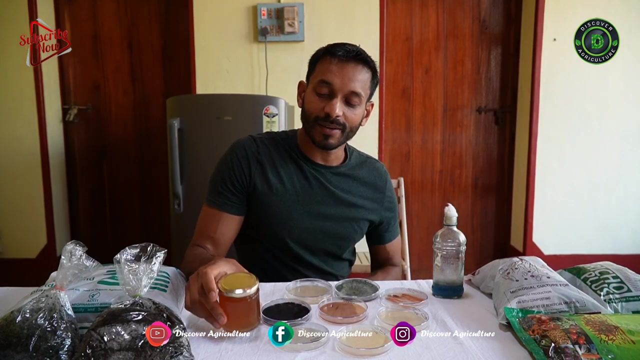 And also the quality of the fruits is apparently improved in the presence of Fracturea, Because it makes the potash more available for the plants. It mobilizes the potash for the plants. So here we have Fracturea. Next up we have in my hand is an inoculum. 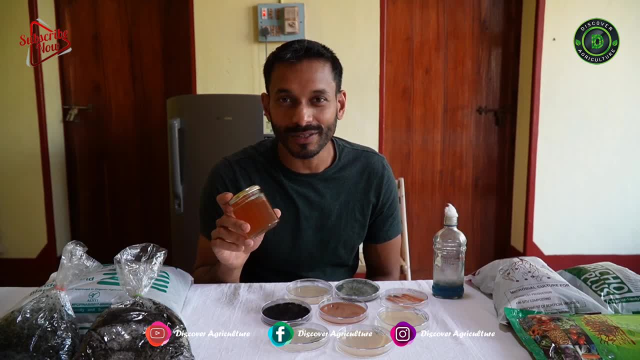 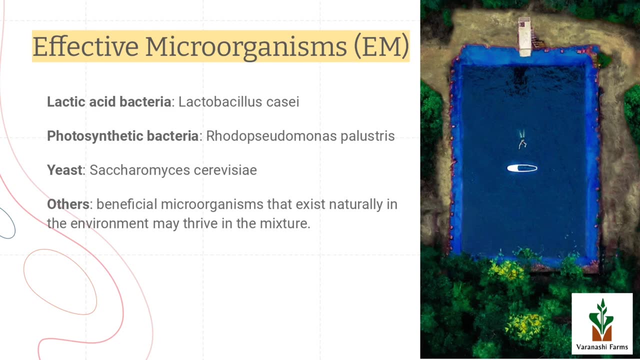 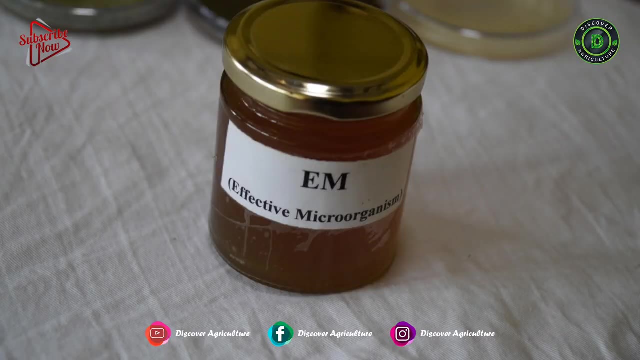 of effective microorganisms. So basically it's a liquid consortium of photosynthetic bacteria, some yeast and also some bacillus species of bacteria. So this is a great degrader of organic matter. So in the presence of effective microorganisms it goes into the soil. 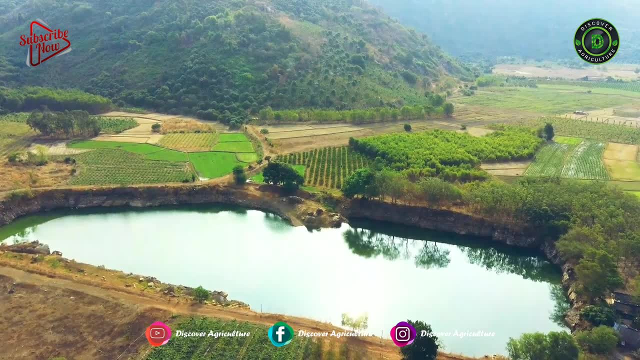 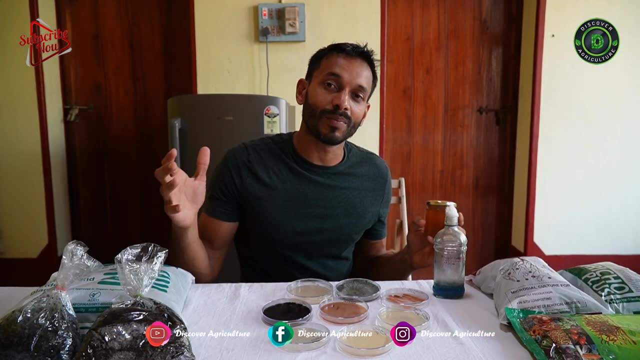 So you can inoculate this into your ponds- irrigation ponds. If you inoculate your ponds every two months, so take up the inoculum, put it in a drum like a 200 litre drum with 4 kilos of jaggery. 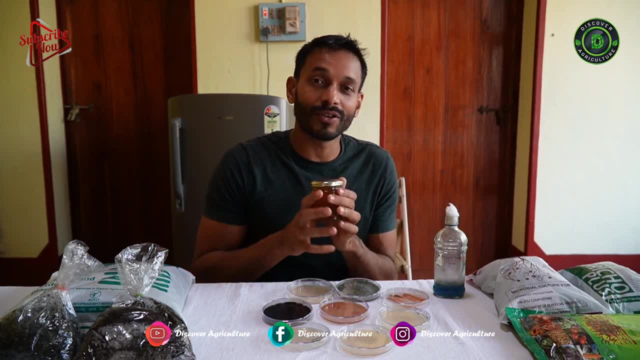 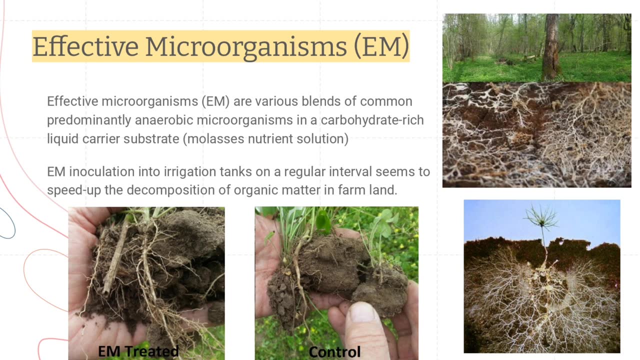 and mix it up. stir it up And you inoculate it to your irrigation pond and then you irrigate it Once it reaches your soil. it helps in degradation of organic matter in the soil. It enhances the root growth and also makes these nutrients more bioavailable for the plants. 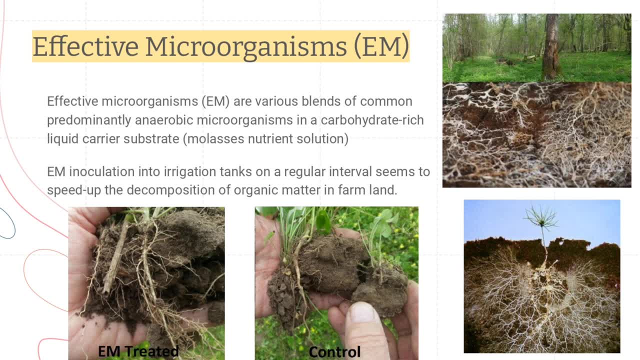 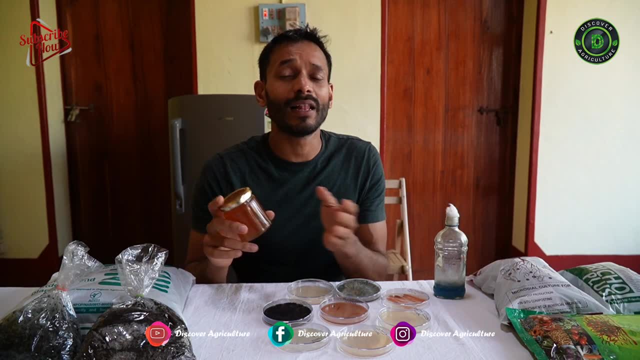 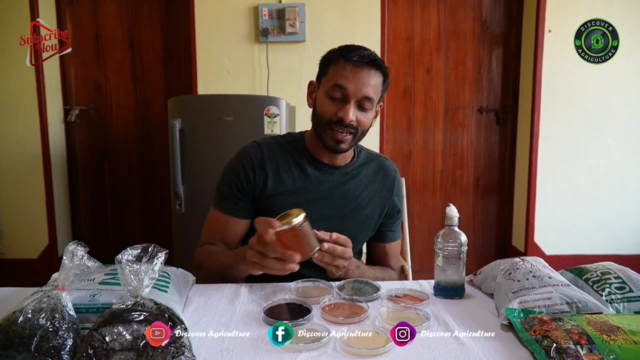 And also another benefit of EM in your pond is it doesn't allow the algae to grow, So the algal growth reduces and then that will help you keep your pond water clean and also your pipe systems clean. So that's EM. So it also goes really well with the other consortium of biofertilizers. 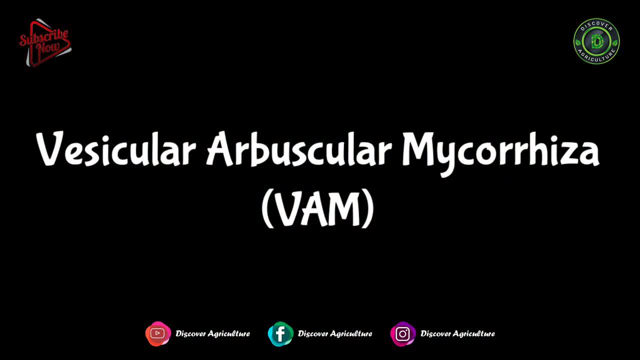 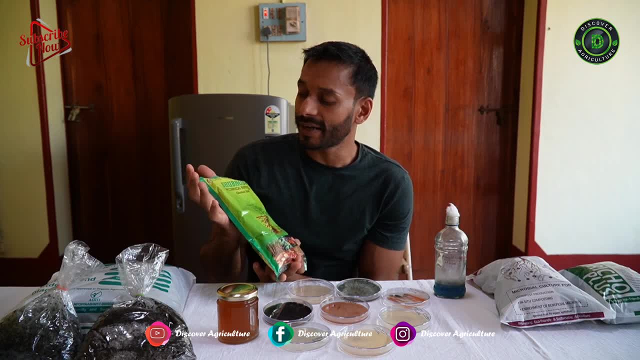 And then we have VAM, vascular or vascular mycorrhizal. There's one called Clomus species, which is produced by Cosme Biotech- Cosme Biotech in Goa, And we use it quite a bit. So what VAM does is 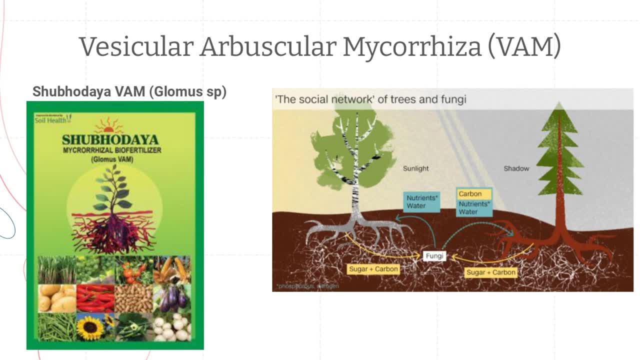 it's a fungal mycelium which connects the roots from one plant to another and also travels widely under our plantation. So, like in the forest, the VAM connects onto the roots and spread across the field, collecting the water nutrients from all different places. 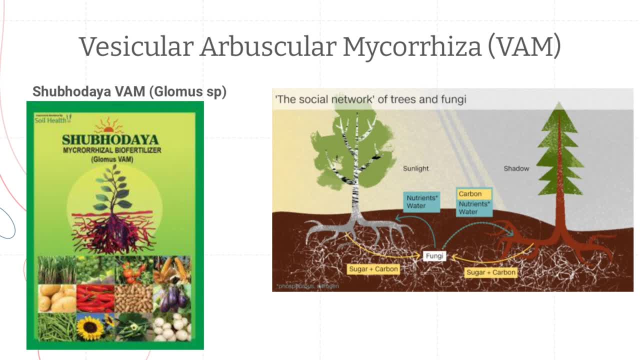 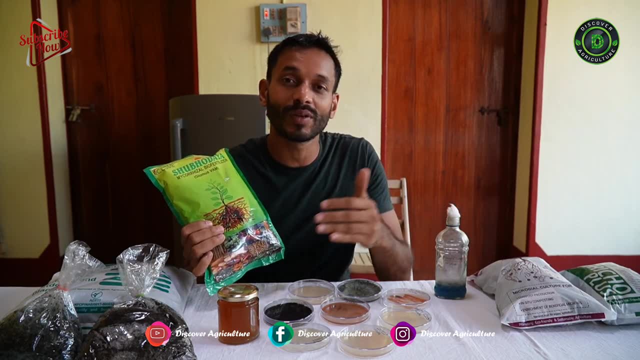 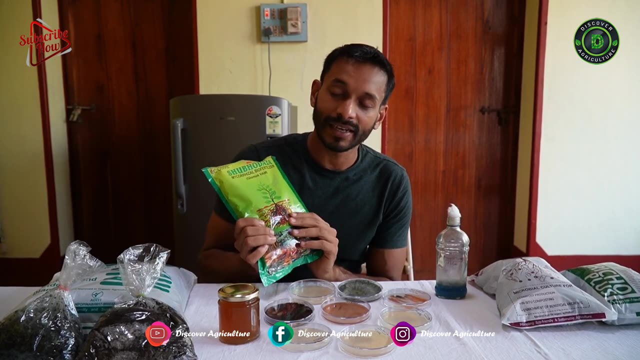 into your plant roots. And also another thing it does is it gathers information from various parts of the field and it gives that information to each and every plant it's connected to, which is all the plants present in your plantation, And say if there is drought coming up. 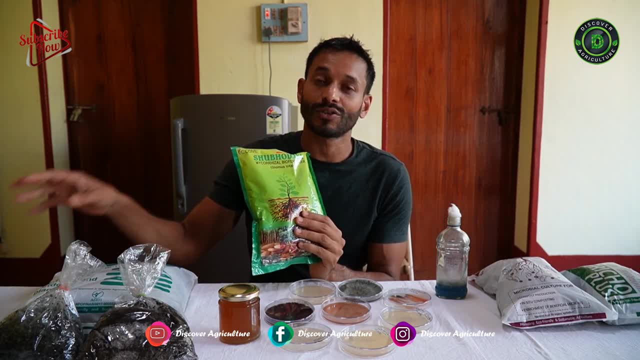 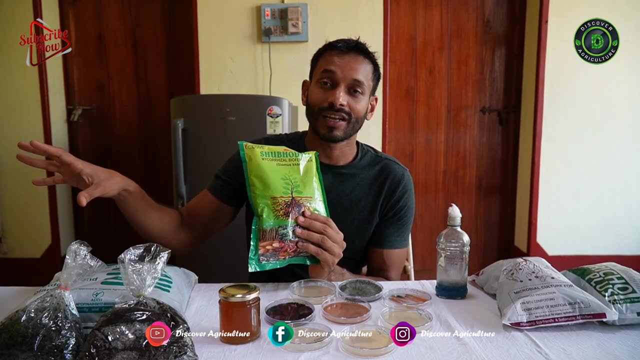 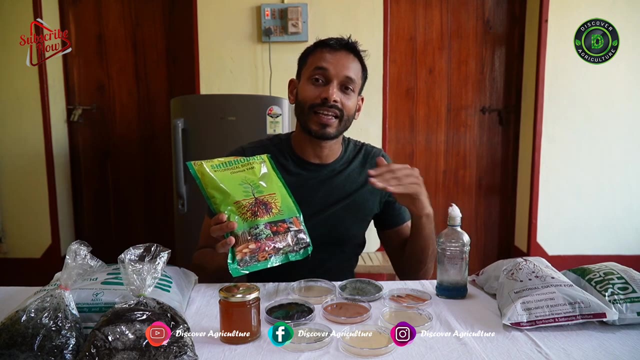 or if there is some epiotic or abiotic stress, like pathogens or some disease coming up with the pathogens, or there is lack of water, there is drought coming up or there is higher salinity. It gives this information to all the plants so that they can prepare themselves. 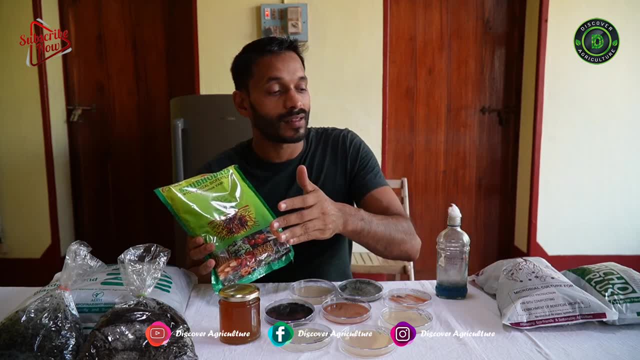 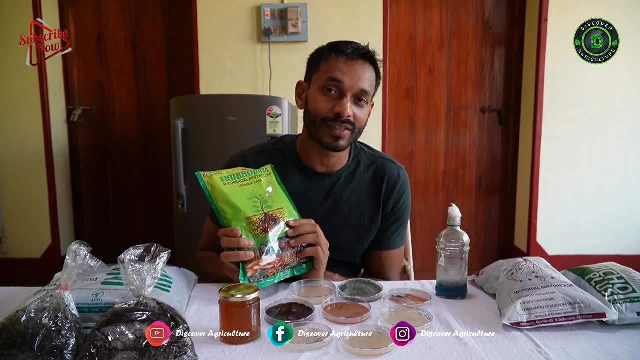 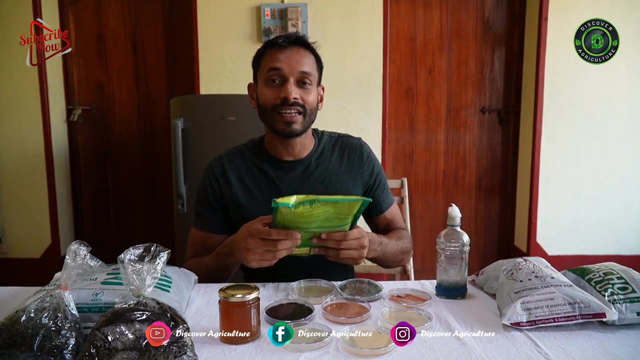 so that they produce phytohormones. The consortium of microbiota around it produces whatever is required for the plants to improve its immunity and its sustainability. So this VAM gives them that information Early on Early warning system we can call it.